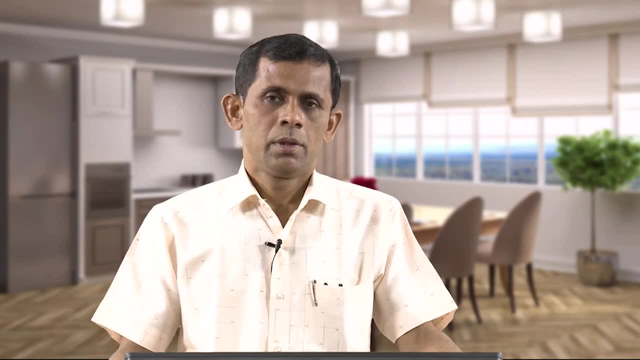 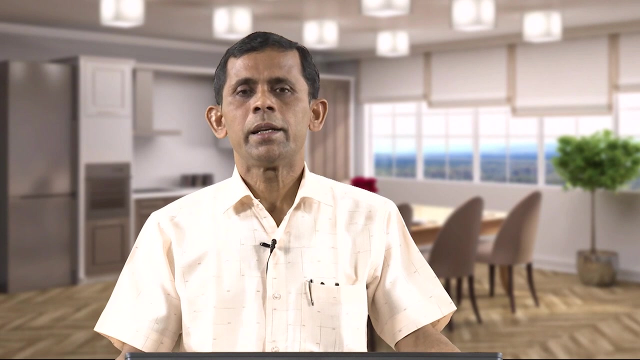 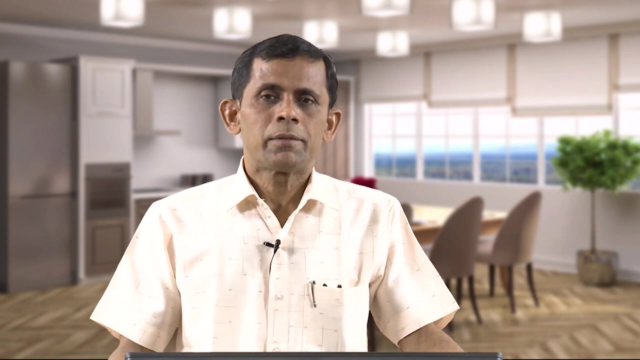 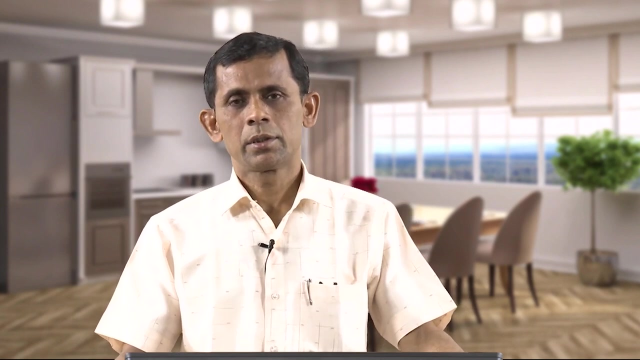 environment are two major concern. due to ever increasing population, urbanization and industrial growth, Pollution generation is increasing day by day around the globe, resulting many disadvantages or health impacts on human as well as difficulties The more we take advantage of different living organisms, and it is changing the climate across. 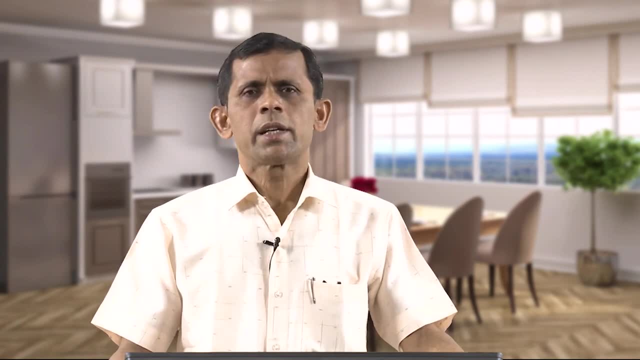 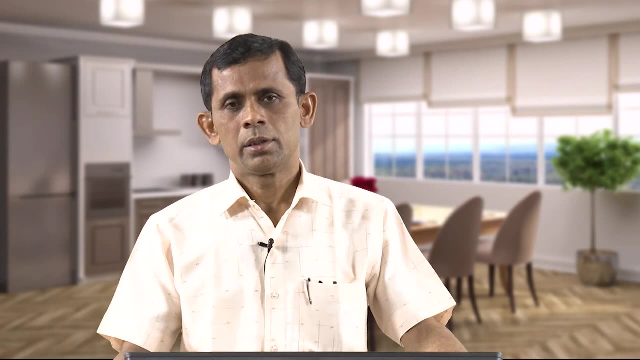 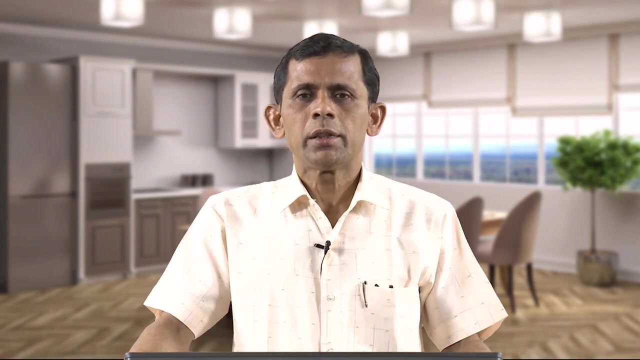 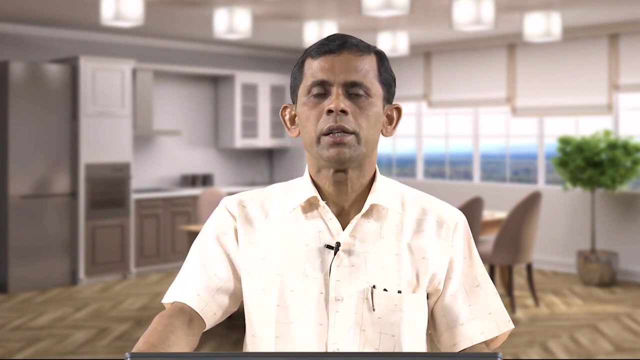 the globe. In short, we can say that in 21st century, our sustainability is under threat. So to ensure the sustainable development of the society, it is very essential to reduce stress report, reduce and control the environmental pollution. 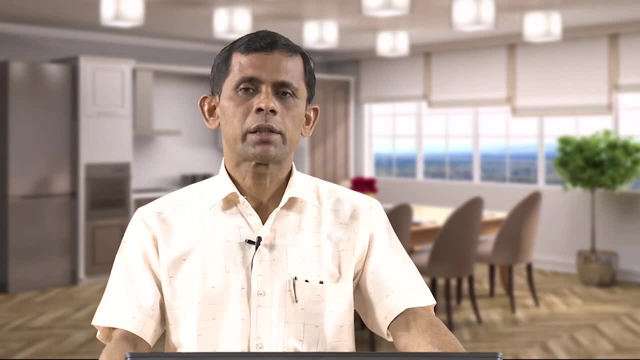 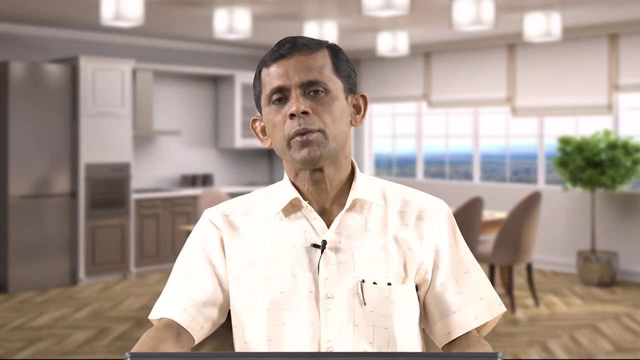 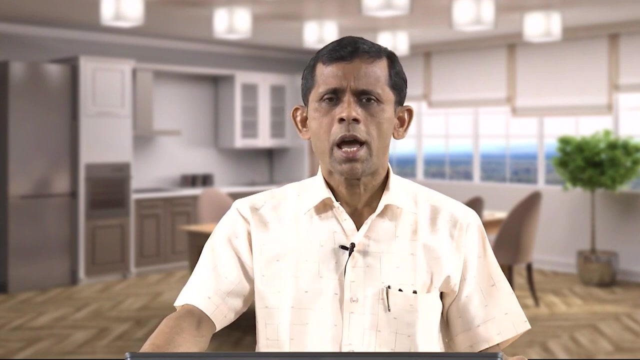 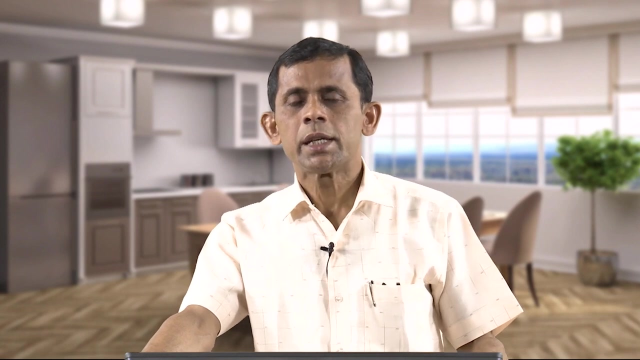 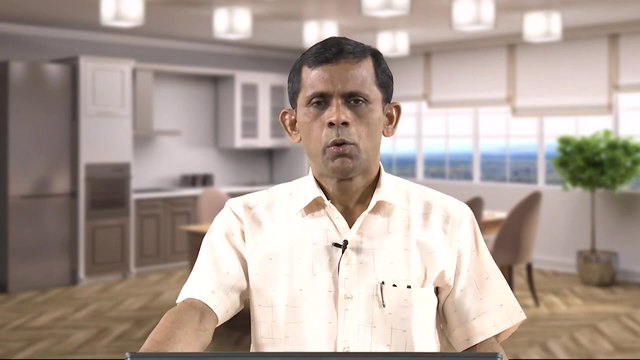 And this can be done if we can create more awareness among the common people and we know the basics of environmental engineering, along with other engineering and science subject. We also have to be more responsible when we are taking some new initiatives so that we will be taking sufficient measures to protect the environment. 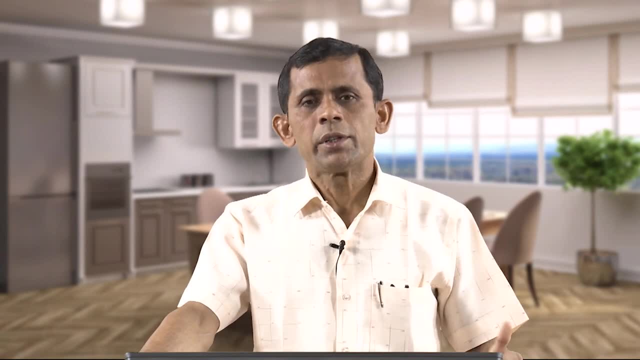 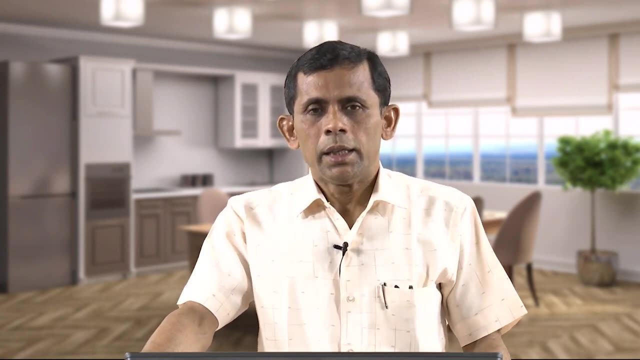 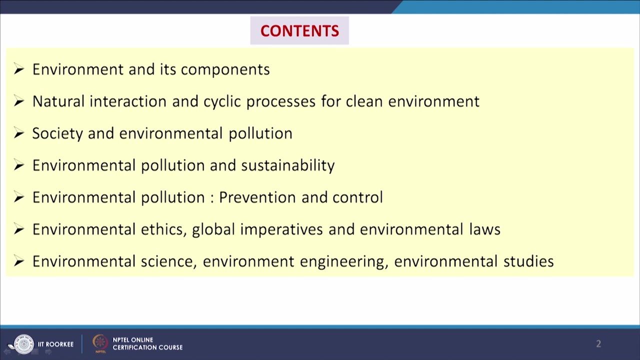 We also need some guidelines, some regulatory framework so that the system works nicely. So in this module we will discuss on this topic, that is, environment and its components, natural interactions and cyclic processes for climate change, Clean environment, society and environmental pollution, environmental pollution and sustainability. 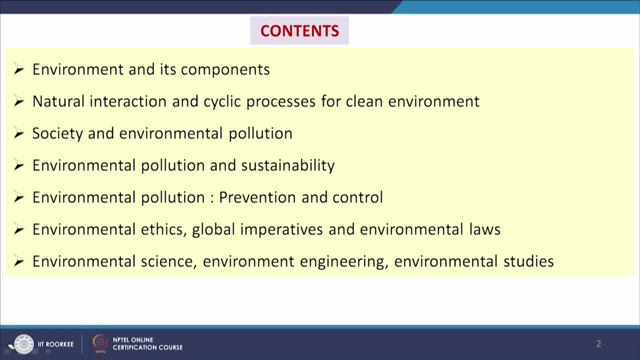 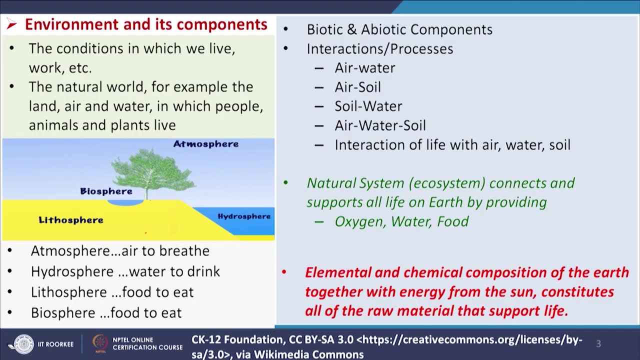 environmental pollution prevention and control, environmental ethics, global imperatives and environmental laws and environmental sciences, environmental engineering and environmental studies. So we will have some overall discussion on these topics. So you see what is environment? So the condition, So the condition. 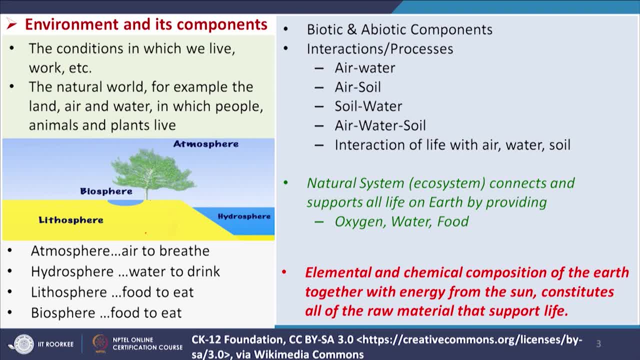 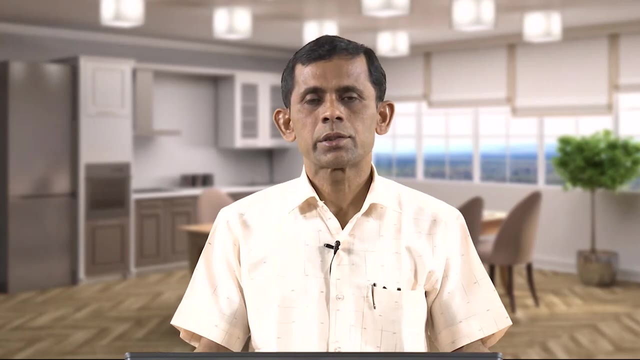 So the condition in which we live, work, etc. that is our environment, or we can say the natural world, for example the land, air and water in which people, animals and plants live. so that is our environment. And if we see the components of environment, then it has both biotic and abiotic components. 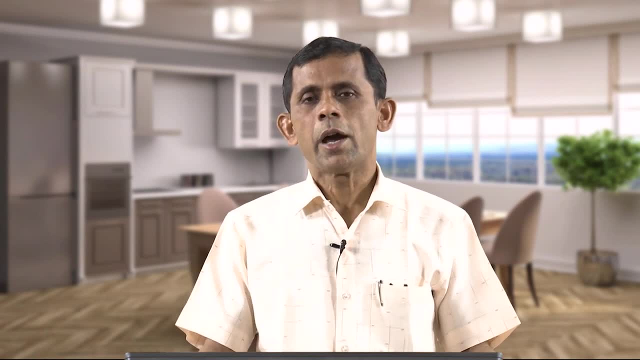 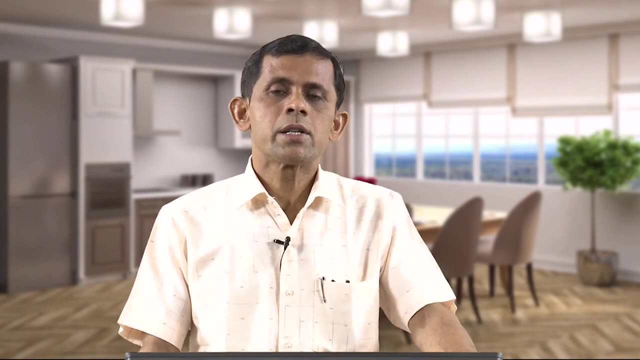 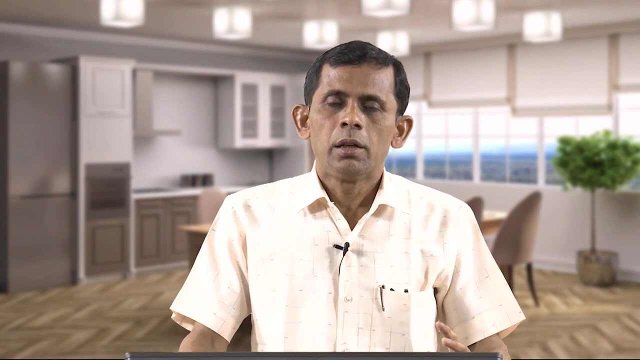 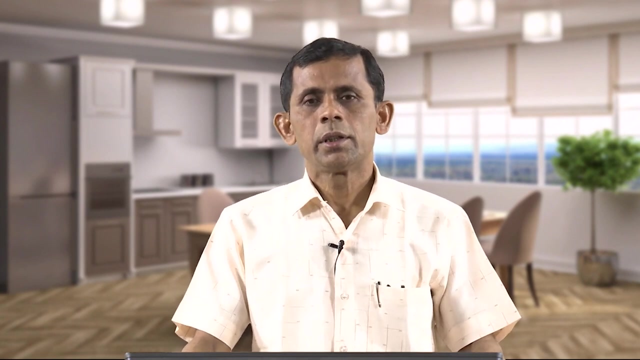 Biotic components are all living organisms And abiotic components are soil, water, air and energy is also an integral part of this environment, or the eco system, These abiotic and biotic components of environment, they have some inter-relation like, say, air-water. 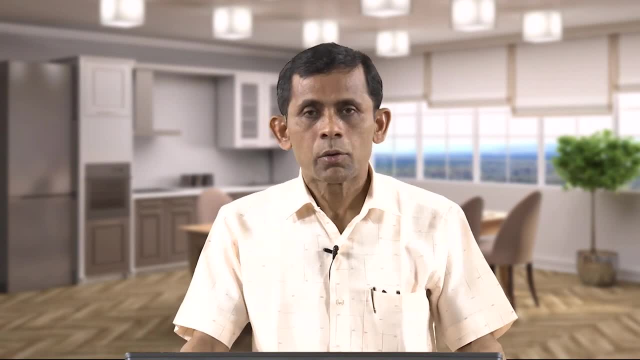 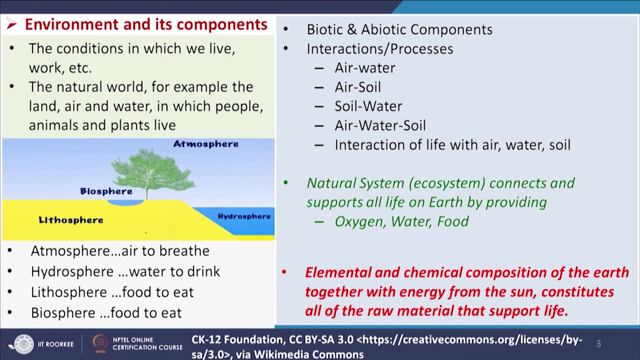 air-soil, soil-water, air-water-soil, water-soil and environmental. So these are the components. Now we will discuss the environmental components, So air-water-soil-water, soil, or interactions with the biotic and abiotic components also. 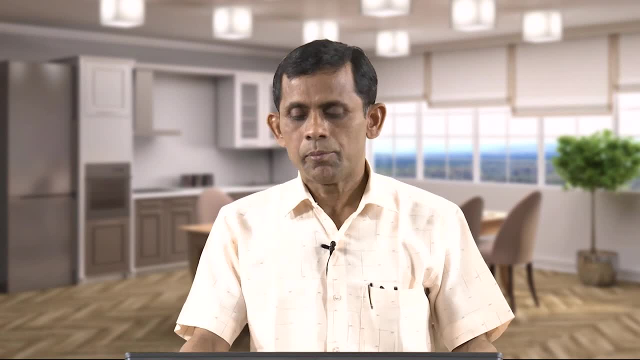 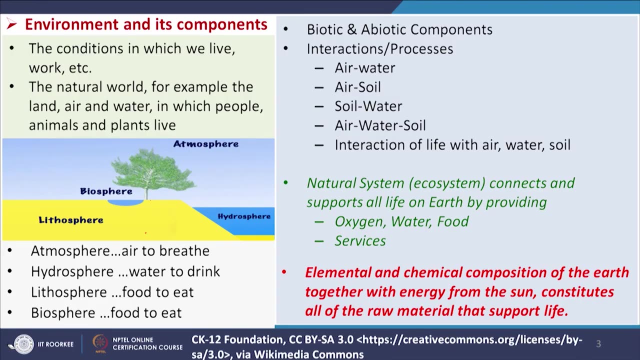 And we know that this natural system or ecosystem that connects and supports all life on earth by providing oxygen, water, food and services, If we see, the environment has four parts, that is, atmosphere, hydrosphere, lithosphere and biosphere. 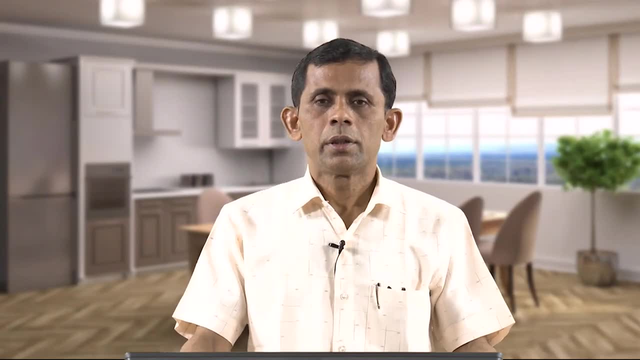 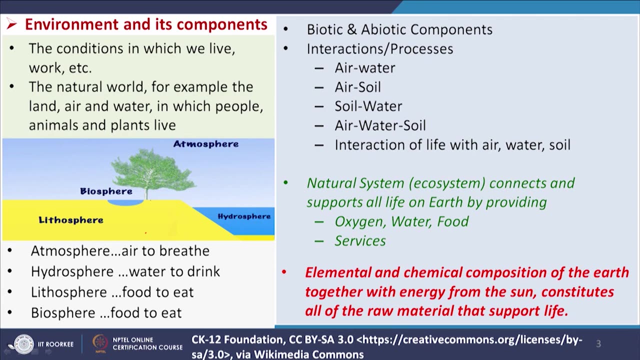 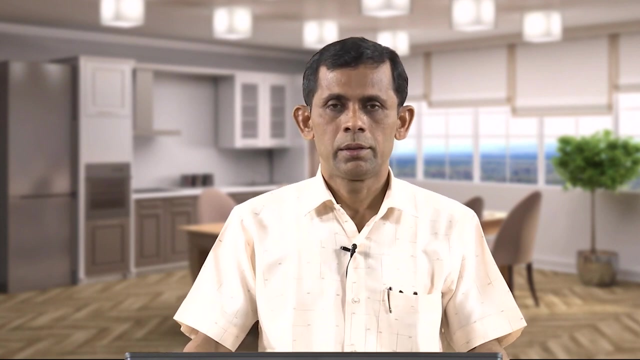 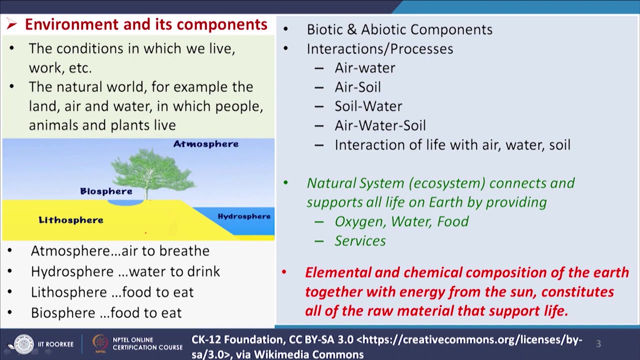 So atmosphere gives us air, lithosphere- that is related to soil and gives us food, and hydrosphere gives us water. and biosphere is that part where living organisms coexist with the non-living elements And elemental and chemical composition of the earth, together with energy from the sun. 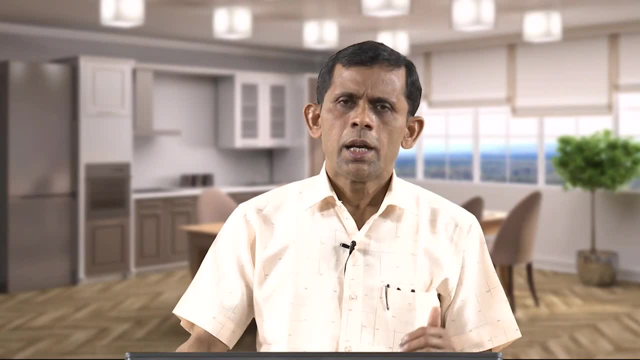 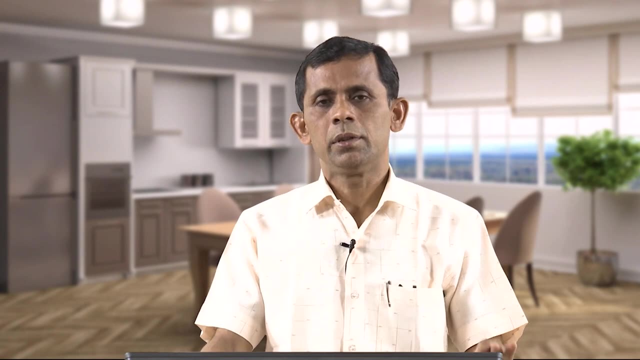 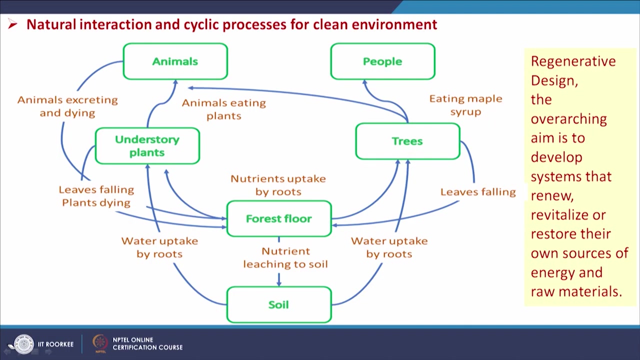 constitutes all of the raw material that support life And in nature, the natural interaction and cyclic processes are available for clean environment. For example, in this figure, if we see, we know that the trees and plants produce food from the sunlight using water and carbon dioxide. 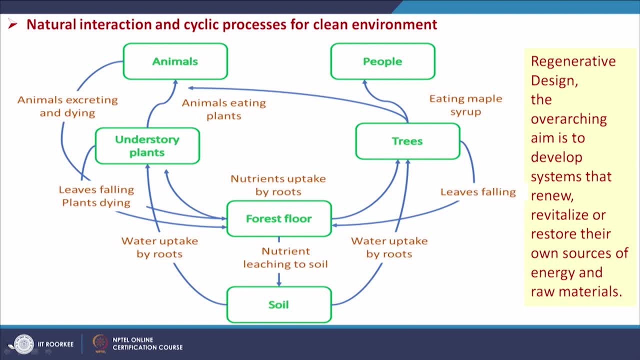 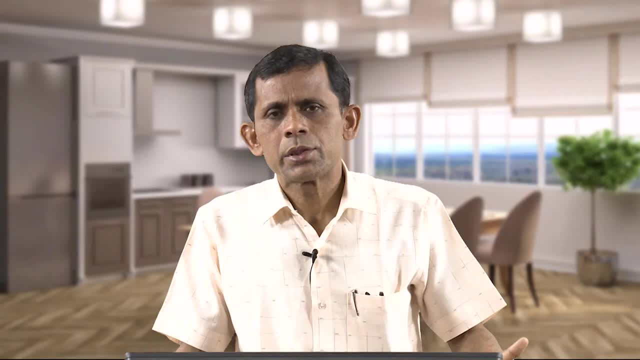 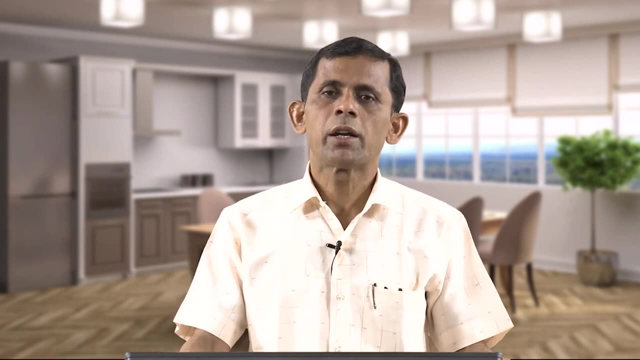 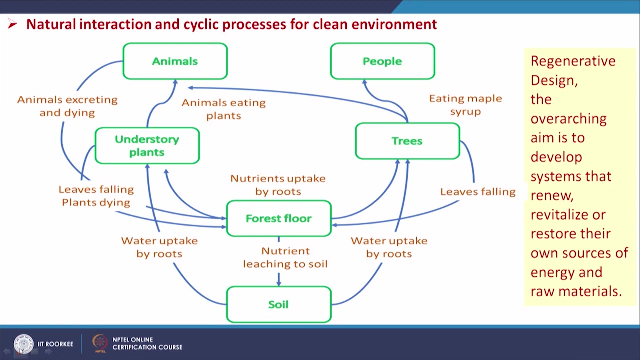 And that is taken up by the other animals, Including the human being, And after the growth of this human being and the other animals, the dead biomass comes into the environment, from where again the nutrients enters into the soil, as shown in this figure. So here this is trees and then plants, and we are. it is people is taking from it animal. 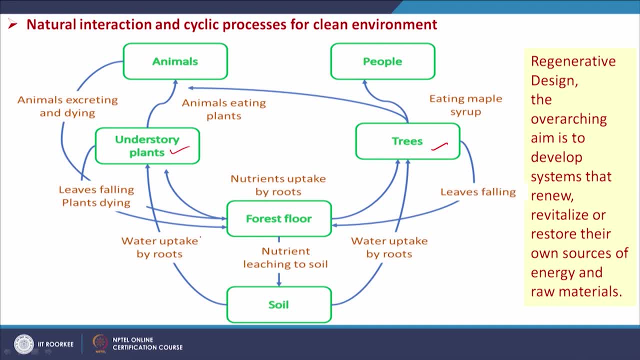 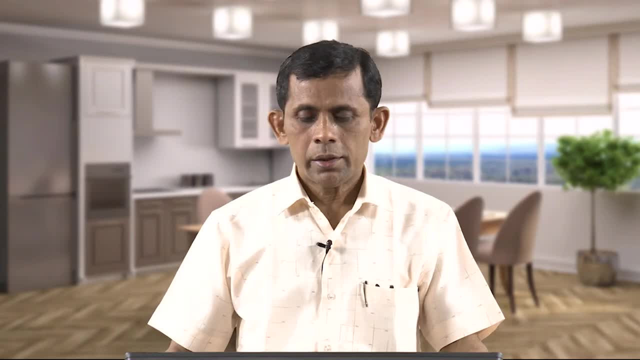 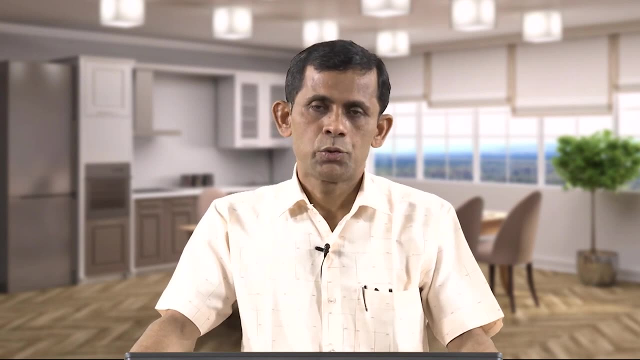 are taking from it the food and they are growing And after that again it is coming to the forest floor. so these are the nutrients, So what we see here, that in environment has some regenerative design. If there is some disturbance, so it can accommodate it and it can revitalize or restore their own. 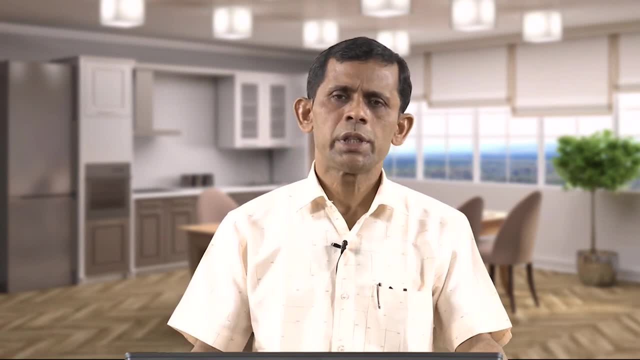 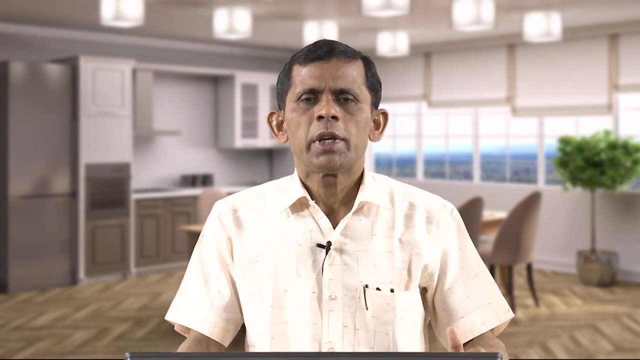 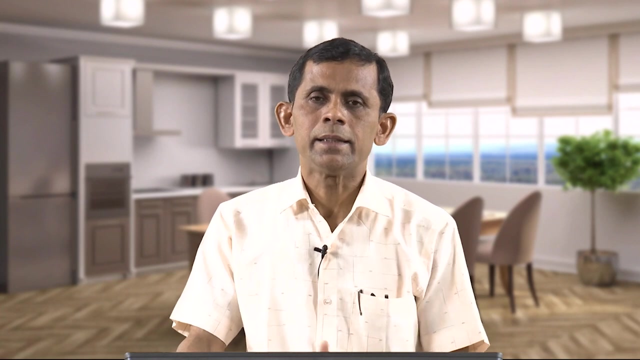 sources of energy and raw materials. This is the beauty of the natural environment, But we have to understand. We have to understand What is happening. due to excessive population growth, Many activities are taken up which are affecting the natural cycle process of the environment. 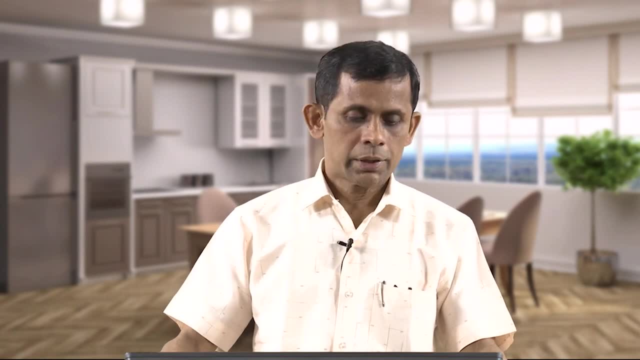 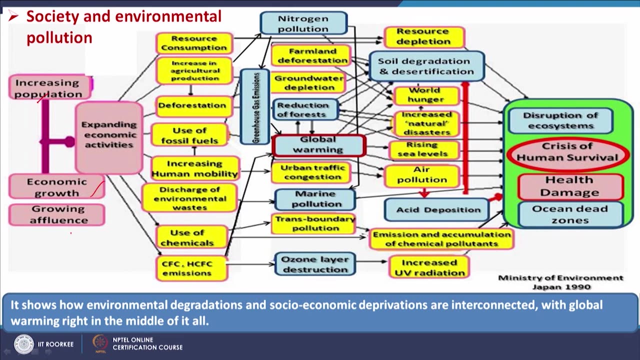 So this slide gives up some idea about it. You see, when we are going for increasing population, so economic growth and growing affluences, That means, you know, the prosperity of the human society. So those are Compiling to expanding economic impacts and which are giving us some activities, like say, 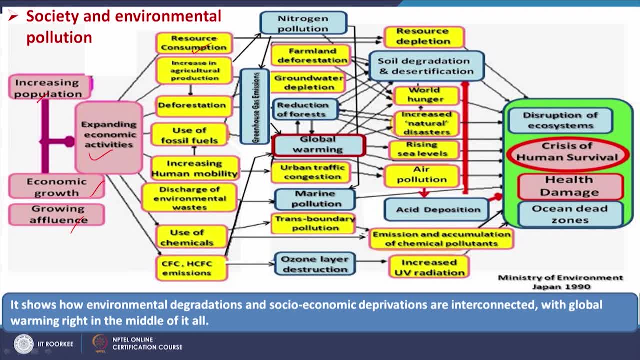 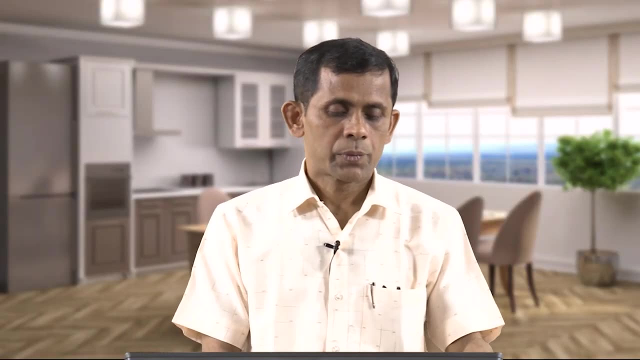 resource consumption, increase in agricultural production, deforestation, use of fossil fuels and increasing human mobility, discharge of environmental wastes and then use of chemicals, CFC, HCFC emissions. So these are the things, Okay. So these are the inevitable consequences of the expanding economic activities. and because 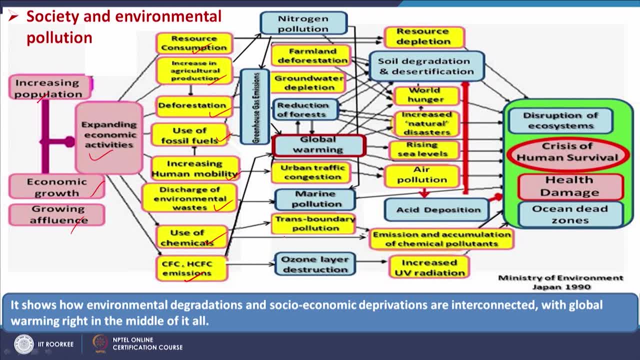 of these activities, we are getting some secondary and tertiary impacts which are interrelated in many cases to each other. For example, say, greenhouse gas emission we are getting, so that is nitrogen pollution we are getting- Okay, So we are getting farmland. 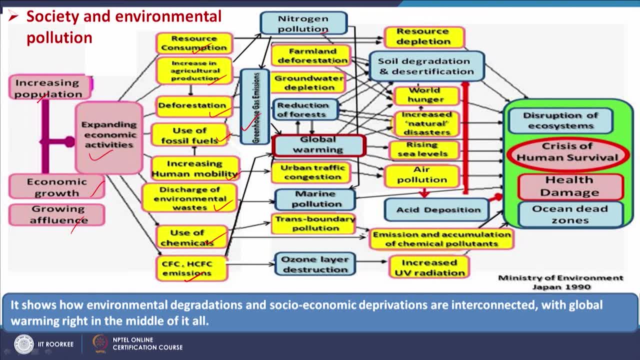 Okay, Okay. Deforestation, ground water depletion, reductions of forests, global warming and then urban traffic congestion, marine pollutions, transboundary polutions, ozone layer destructions- All those things are some impact of these activities And another impacts are also, you see, resource depletion, soil degradation and desertification. 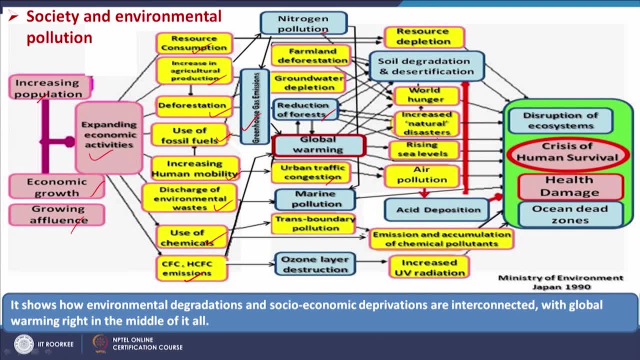 wild hunger, increased navigating toавast, Deforestation, groundwater depletion, reduction of water usage, global warming and then urban traffic congestion, marine pollution, transboundary pollution, ozone layer destruction- all those Increased natural disasters, rising sea levels, air pollution, acid deposition and emissions. 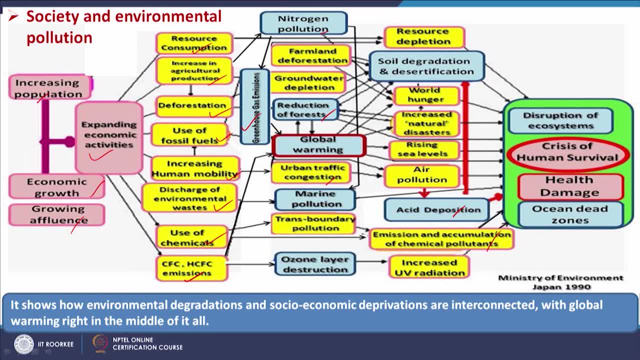 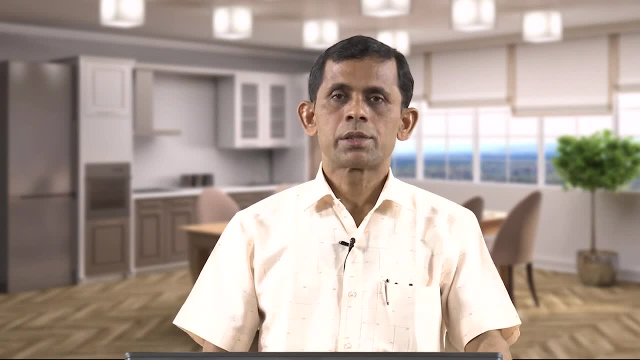 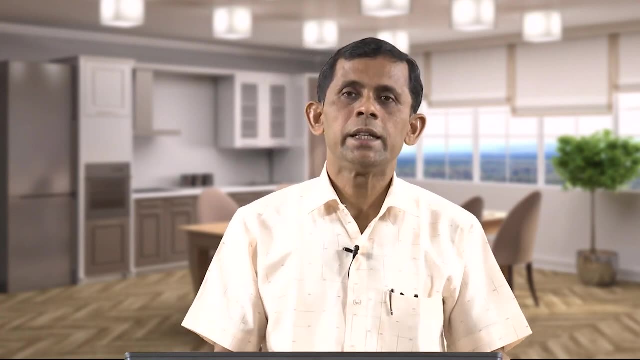 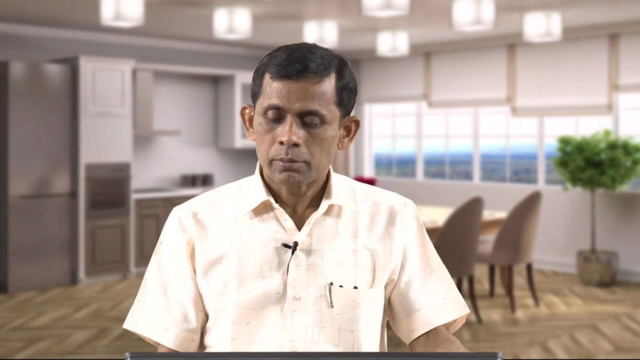 and accumulations of chemical pollutants and increased UV radiations. As a whole, the human survival is under threat, but this is a crisis of human survival, So the human activities are responsible for the destruction of the cyclic process which is available in the nature. as a result, the ecosystem is being degraded and our environment 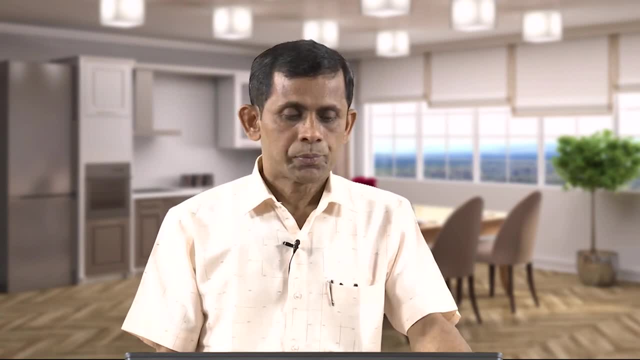 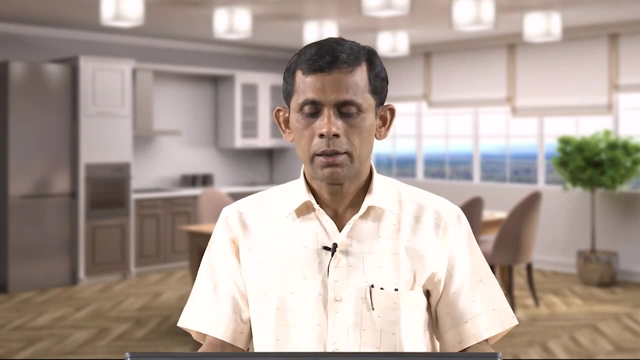 is being polluted. Now we will see how the wastes and pollutions are generated. what types of wastes are there? So, if we classify them, If we classify the wastes, we can classify it in based of hazardous and non-hazardous. 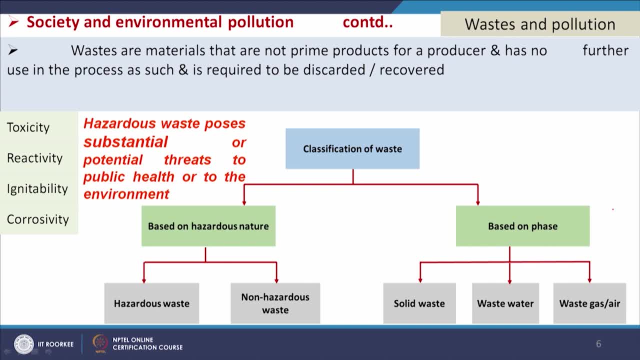 nature and they are based on phase, also, So hazardous and non-hazardous. we know that the wastes or pollutants which are having certain properties like, say, toxicity, reactivity, ignitability, corrosivity- any one of these or any combination are, all are having the hazardous characters and those wastes or those 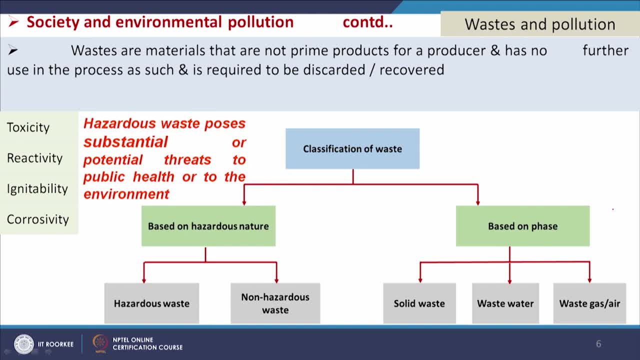 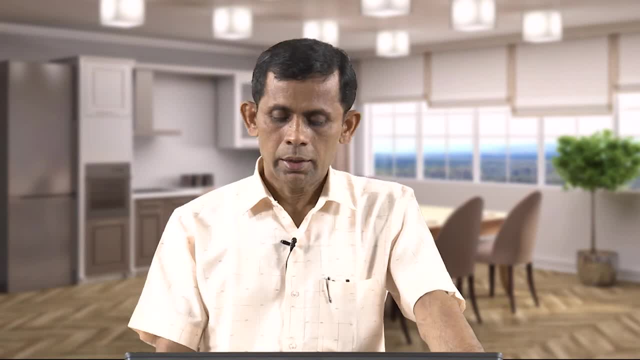 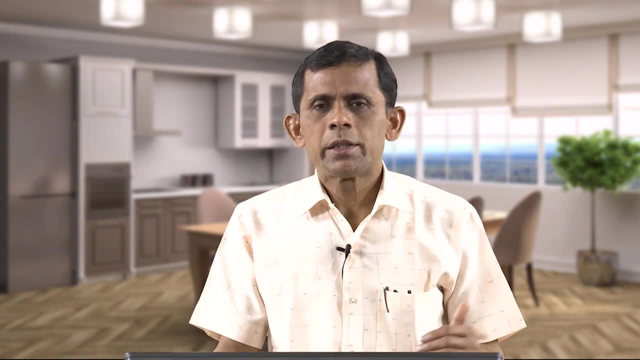 pollutants are hazardous pollutants or hazardous wastes, So it is a very high risk waste and non hazardous. those are not having those characteristics and based on the phase, the waste or pollutants can be in solid waste water or in gas phase also, And we see the economic development influences the waste generation. this table shows us some. 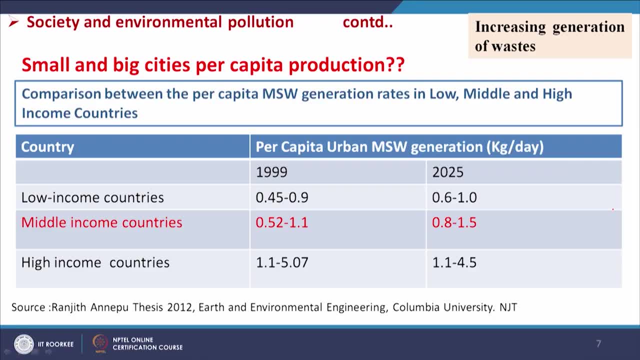 information, that is, low income countries, middle income countries, high income countries have the per capita urban MSW generation is increased during past few years, 1999 and it is predicted in 2025.. So we see that low income countries 0.45, 0.92. it is coming to 0.6 to 1.0, but for middle 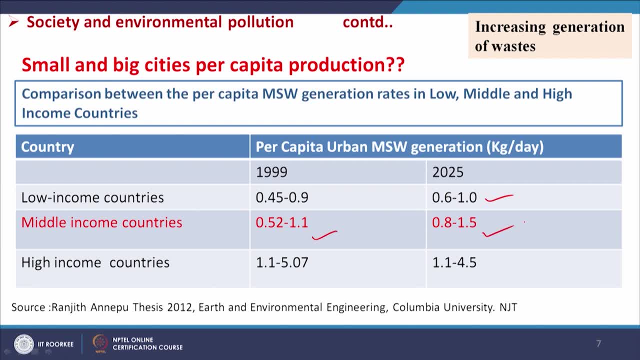 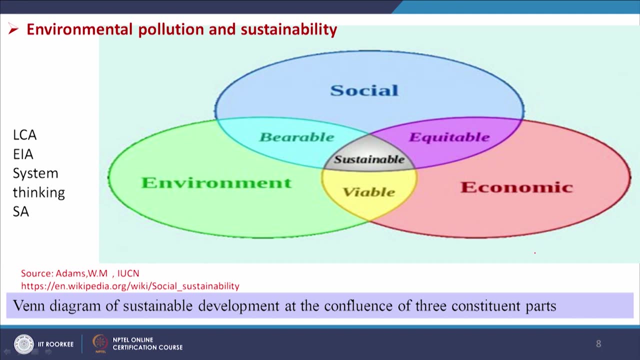 income 0.5 to 1.1 to 0.8 to 1.5 and for high income countries 1.1 to 5.07 to 1.1 to 4.5.. So what we see? that with economic development, the waste generation is increasing gradually. 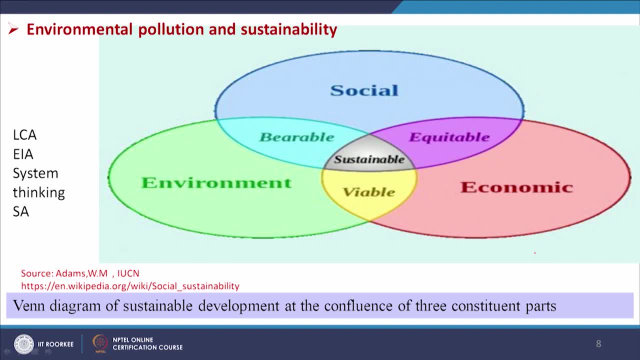 and, due to this, our existence, the sustainability is under threat. We know, to make a system sustainable, or to make a process sustainable, it has to be economically viable, it has to be environmentally bearable and it has to be socially equitable. So this is. 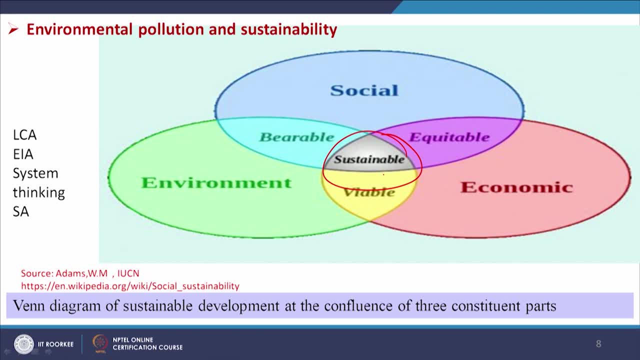 So this is our sustainable this zone. so since the environment is disturbed due to the pollution, So we cannot attain the sustainable society, although we can achieve the economic target and social equity, but still the system cannot be sustainable. to make the sustainable, environmental sustainability is essential. 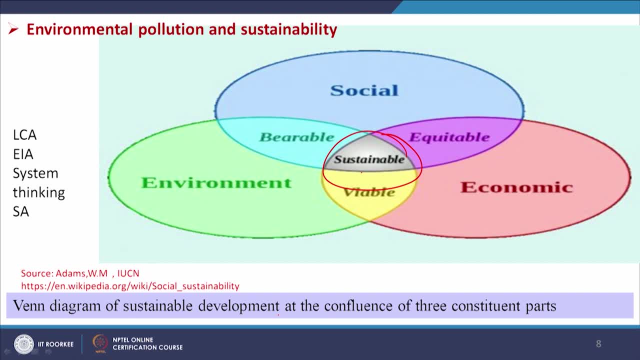 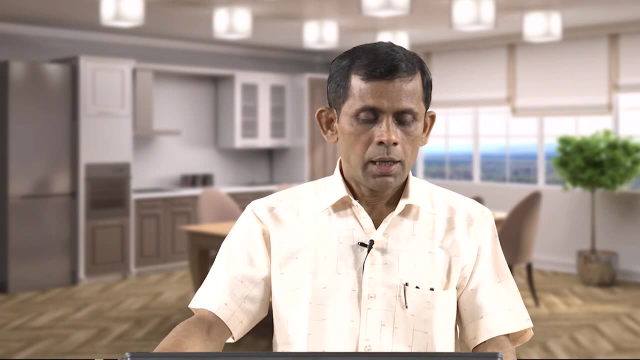 And for that we have to learn, We have to do something. what are those we can do? the LC analysis, life cycle analysis of any processes or any system, and we can take a decision for its modifications, for a changing changes, etcetera, And then environmental impact analysis. that is also practiced, and system thinking can. 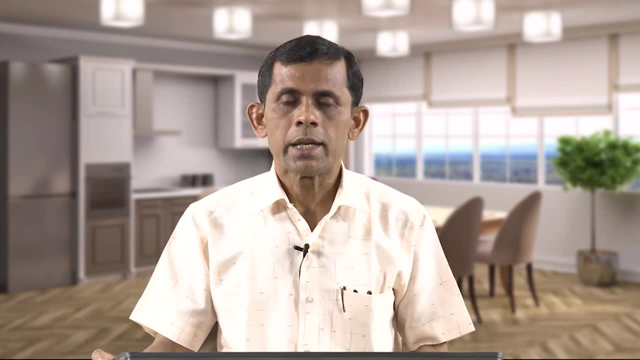 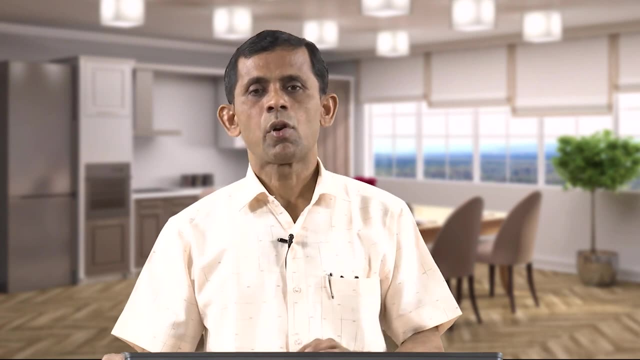 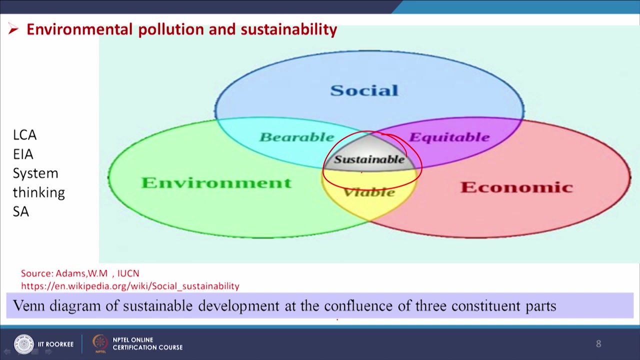 be implemented for any new initiatives, so that we will think about the every stakeholders, not a linear thinking, and the cause and effect relationship And sustainability analysis will also be tool that has to be implemented for any process to analyze or new initiatives, the what will be the impact to the environment, so that 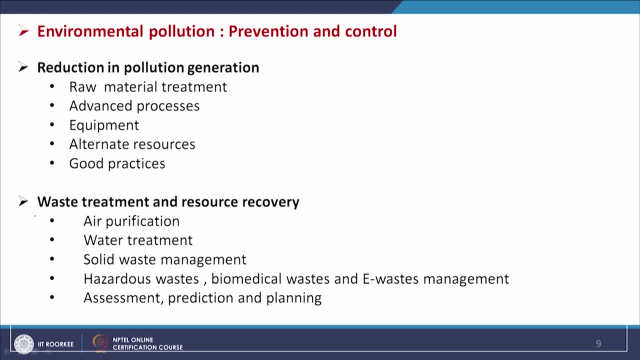 the environment can be safe. Now we will be talking about the prevention and control of pollution. You know, we know very well that for any problem, prevention is better than cure. So our first approach Will be to prevent the environmental pollution, so that the more pollution is not generated. 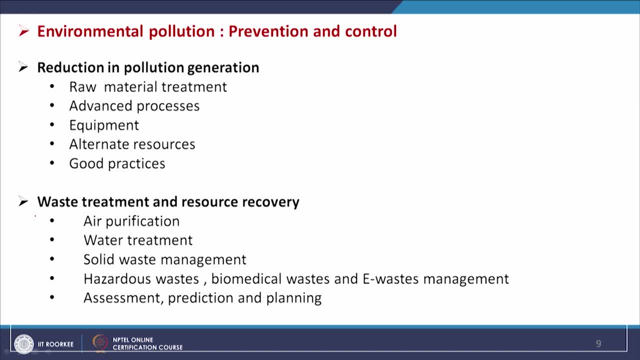 and the second step: if some pollution is generated then we can develop some control strategies and methodologies to control the pollution. So that way prevention and control can help to improve the environmental quality. So, how it is, show the prevention- that is, reduction of pollution generation, that we can do by raw 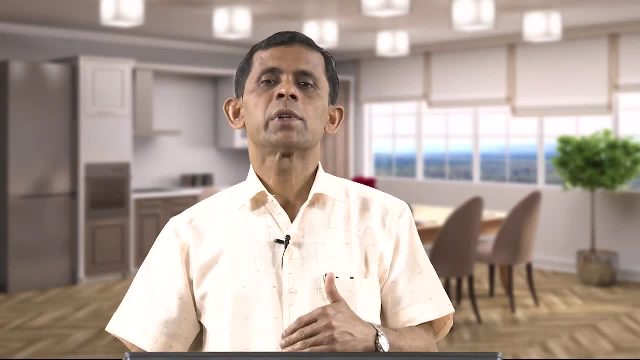 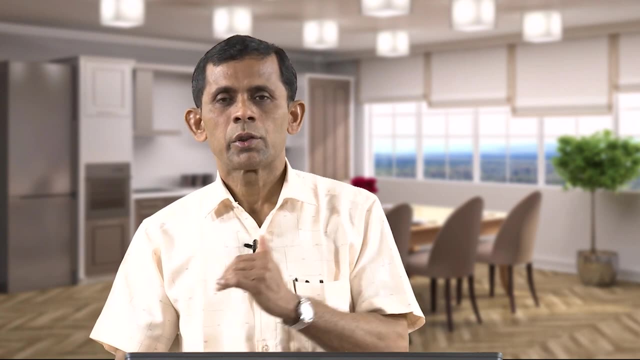 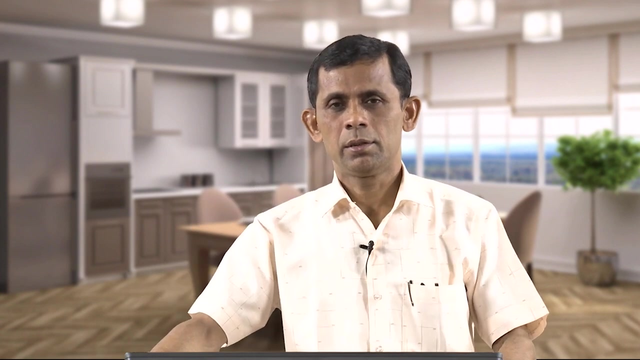 material treatment. So when we are using a process, for example, say coal combustion, we are using flue gas and then it is used in a thermal power plant for electricity production. In that case if we remove the sulphur from the coal prior to its application, then shocks 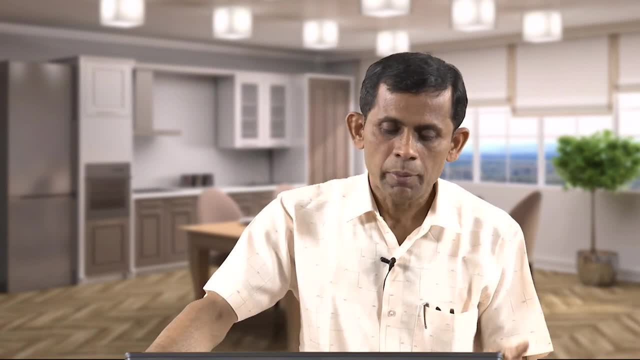 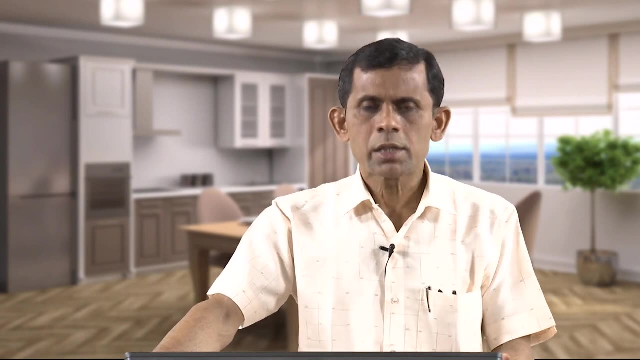 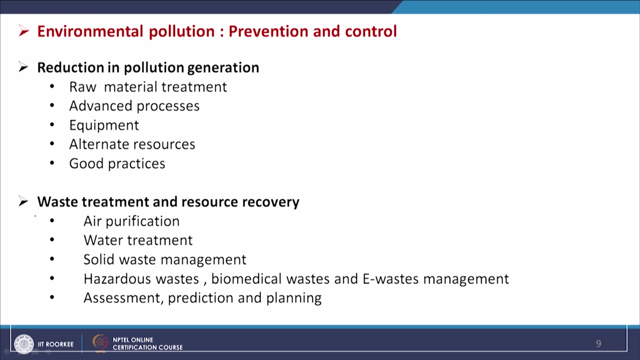 emission will be reduced, so environment will be safe. So raw material treatment is an step which can help us to reduce the pollution generation And advanced processes. we can use some developed processes so that it will be able to generate less pollution to achieve or to give the same amount of work to perform the same job. 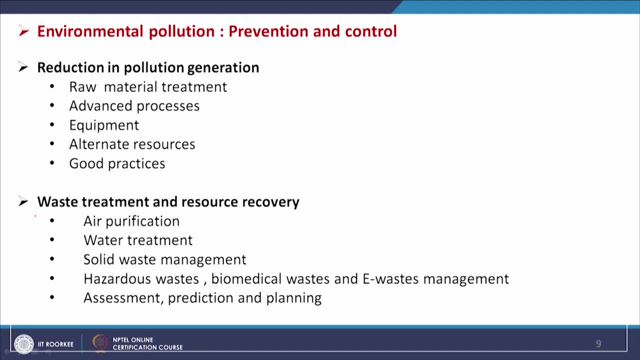 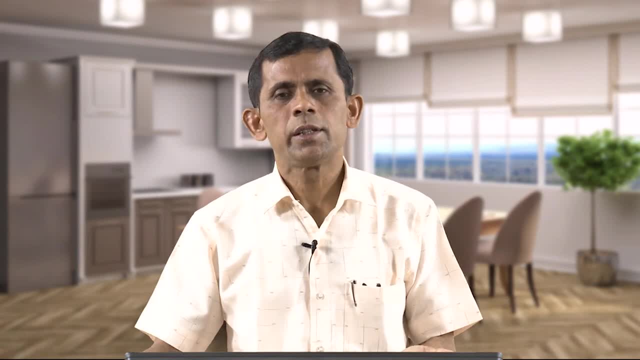 Like, say example, say one is a conventional combustion and another is your oxy fuel combustion. So in oxy fuel combustion we will be using oxygen in place of air, so the carbonaceous material will be producing flue gas which will be rich in carbon dioxide. 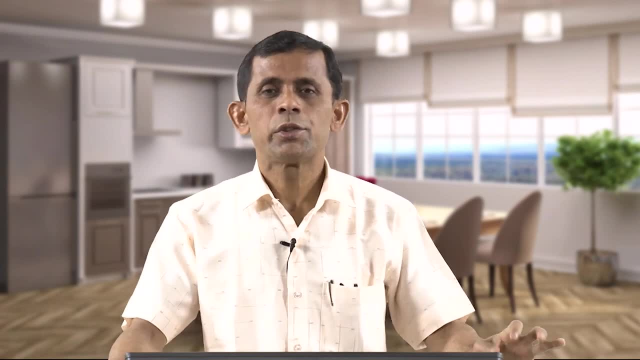 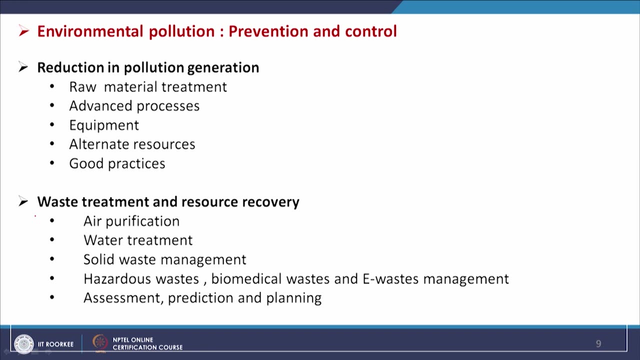 So separation of carbon dioxide and its sequestration will be very easy, so it will not come into the environment And equipment. we can improve the equipment like, say, fixed bed reactor combustor to fluidized bed combustion reactor or combustor in by the modifications in the equipment we are. 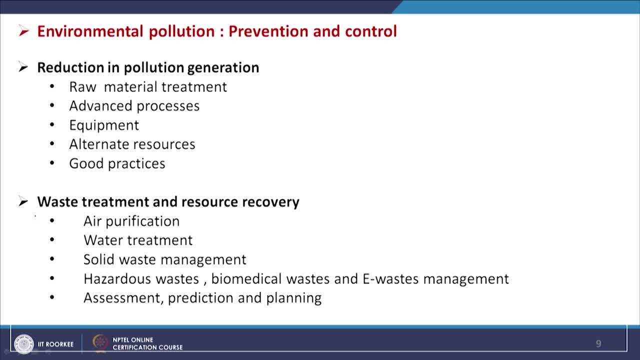 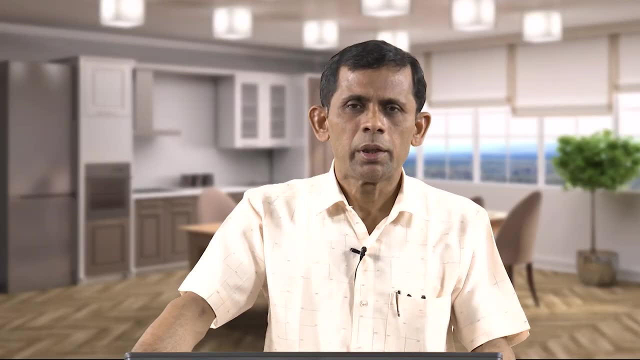 able to reduce the pollution load to the environment And alternate resources like, say, coal, petrol And natural gas we use for the production of electricity, which are creating large number of pollution into the environment. we can reduce its use. we can use the renewable energy. 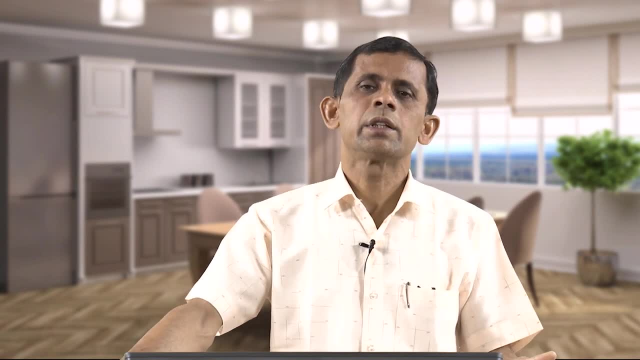 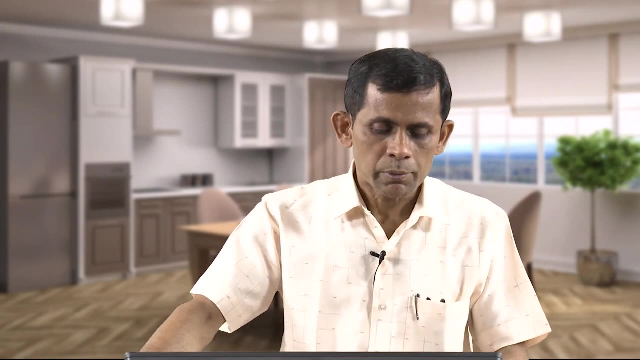 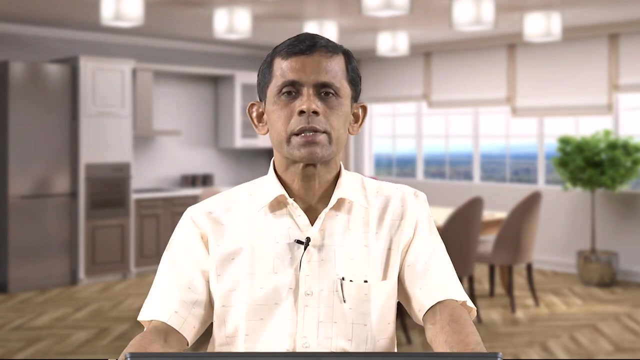 resources like solar energy, hydro energy, etcetera, So that our energy production will be achieved but environmental pollution will be less. so that way also it can be possible. and good practices, You know, by applying good practice also we can save good amount of energy losses. So we are when. 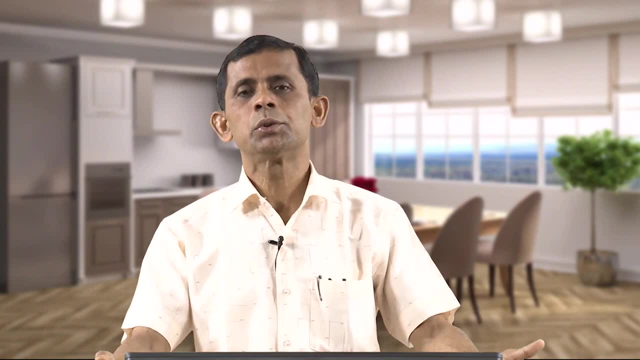 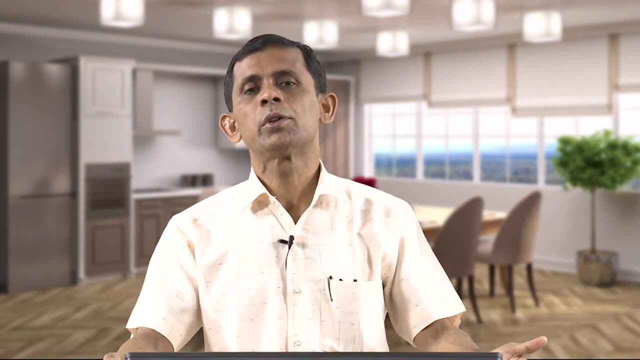 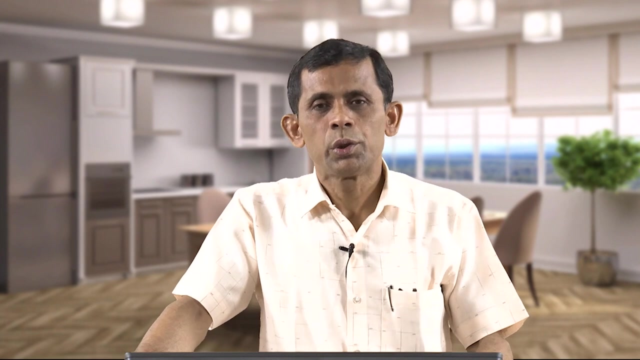 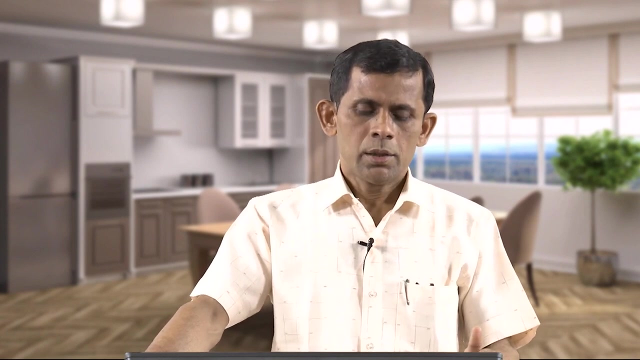 we are able to save energy losses. at the same time, we are able to maintain or reduce the pollution generation during the production of that amount of energy in a thermal power plant. Ultimately, we are able to reduce the pollution load to the environment. Now, waste treatment and resource recovery. this is another aspect. you know when we are 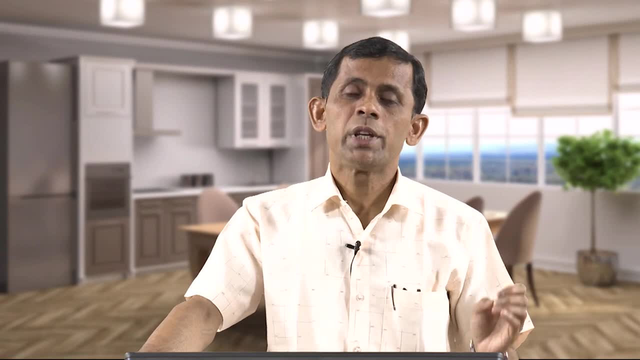 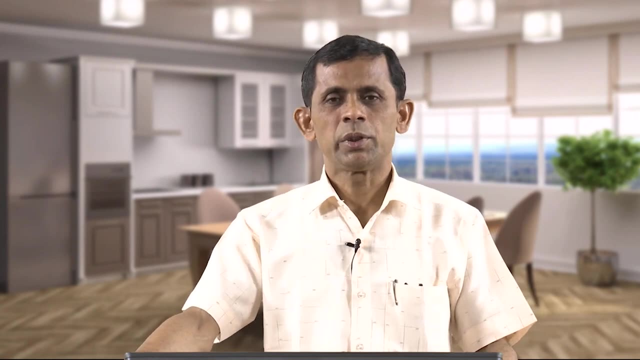 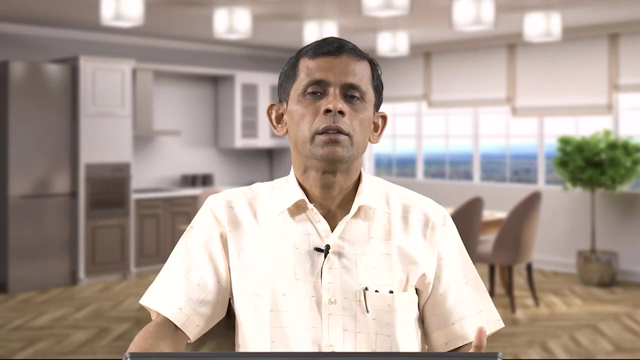 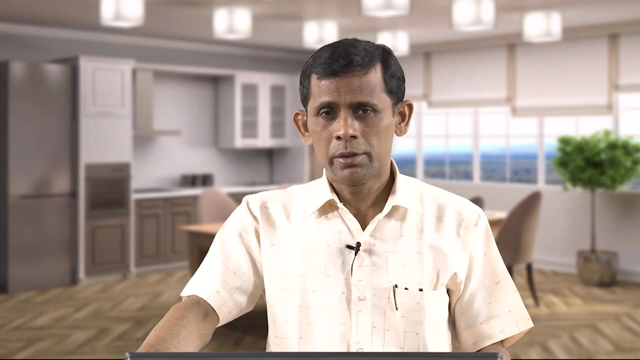 not able to prevent, then pollution is being generated. we have to treat it and we have to recover valuables from that waste stream. So this is the latest research area: the many people are working the waste to wealth, this concept. So here we can work on the air purification, we can work on water treatment, we can work 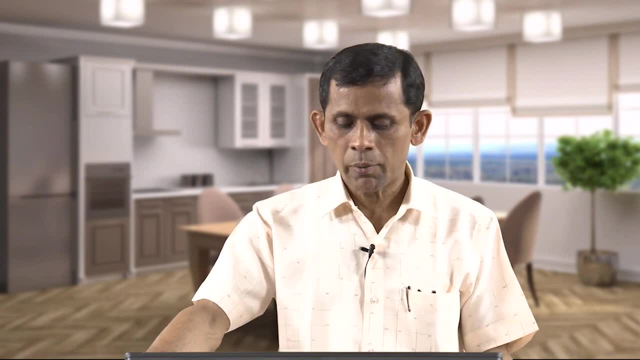 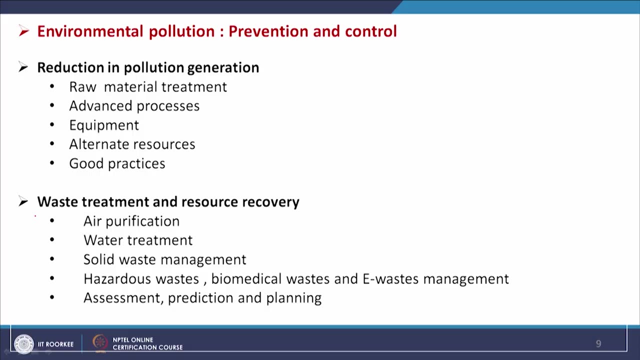 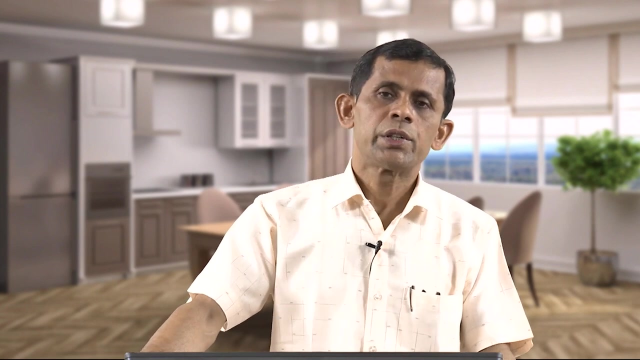 on solid waste management. we can work on hazardous waste, biomedical waste, e-waste management and we can work on assessment, prediction and planning. So these we will be discussing in subsequent chapters. regarding this all control aspect, or treatment and management aspect, Apart from this, we need: 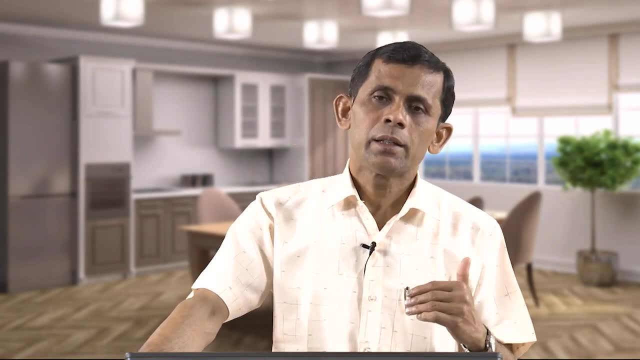 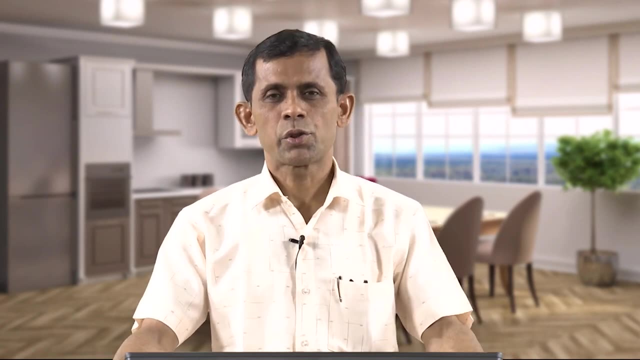 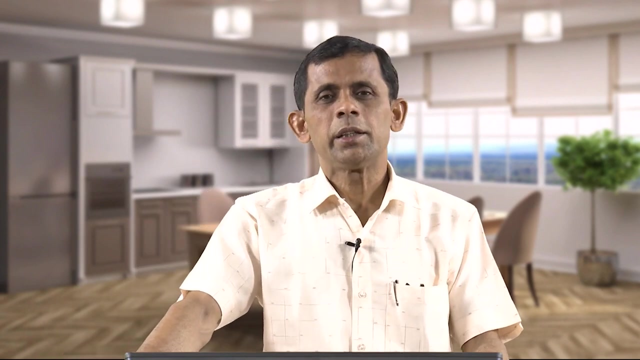 Assessment of the pollution, we can be in a position to predict what will be the pollution after 10 years, after 20 years, after 5 years- long term and short term- and accordingly I have to take a planning or decision. So those things are very, very important. So for that, 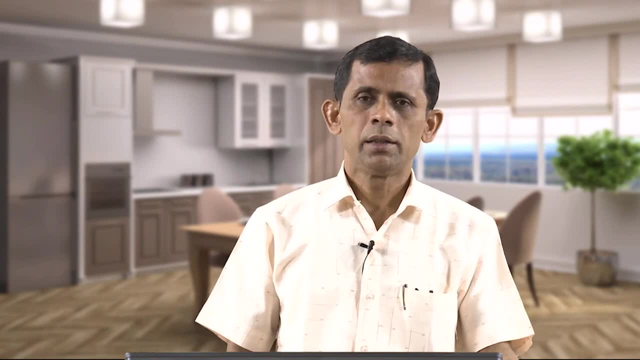 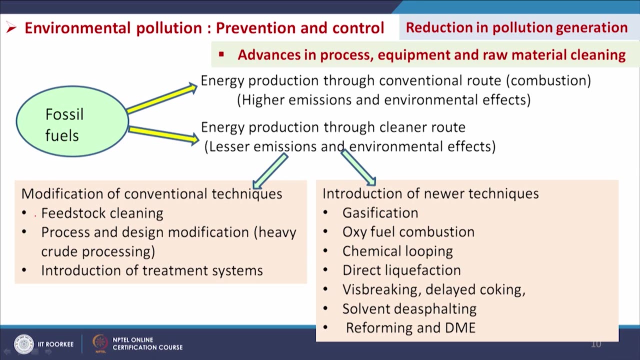 we need to understand the principles of environmental engineering and sciences. Now I will give you some Example here. this slide: that is reduction in pollution generation. already we have discussed also that energy production through conventional route, that is combustion route, it gives up higher emissions and environmental effects. But if we go for energy production through 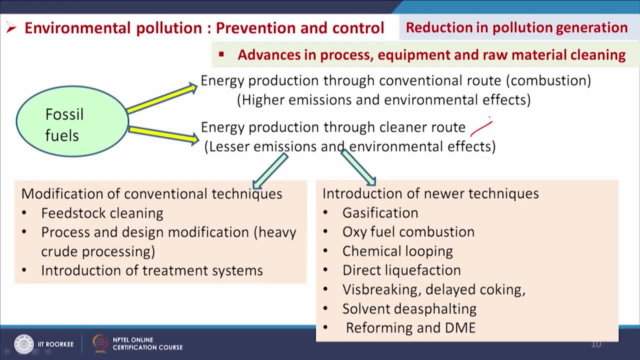 cleaner route, that is, lesser emissions and environmental effects. and cleaner routes can be, you know, modification of conventional techniques or introduction of newer techniques. I have given you some few examples Here. we are having some more examples for, say, modification of feedstock, modification of conventional techniques like, say, feedstock cleaning. I have already discussed process. 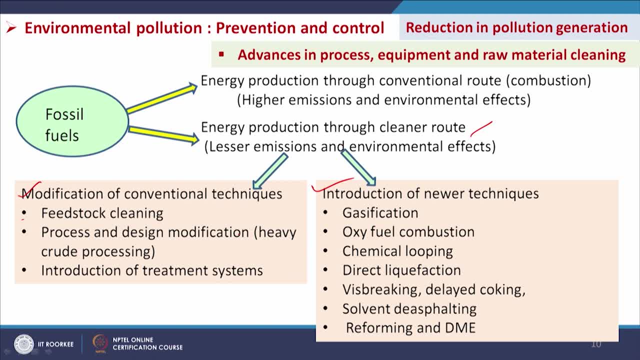 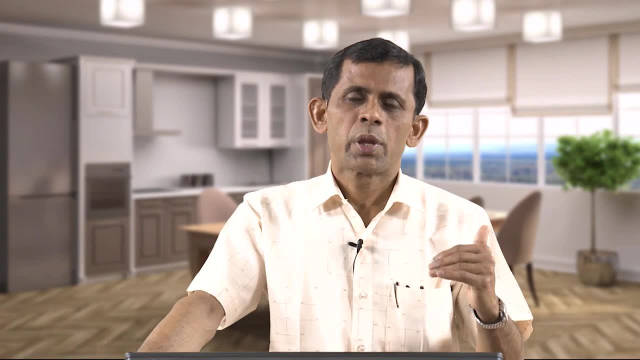 and design modification. heavy crude processing, that is one example, another example. So crude petroleum, crude, which is taken out from the interior of the well, So then dilution is made and then it is transported. So so another approach is that that if the crude is heavier, then transportation is becoming difficult. we have to use more energy for its transport, we have to more diluent for it and ultimately more pollution. But if we process to some extent this heavier crude at the production site and transport it, then it may be possible. 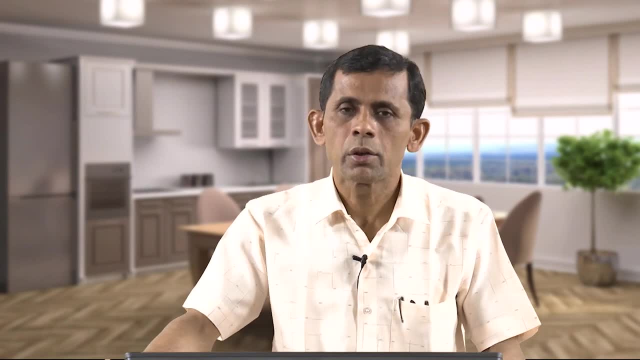 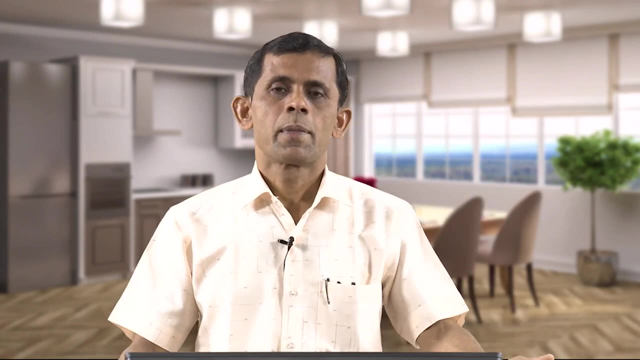 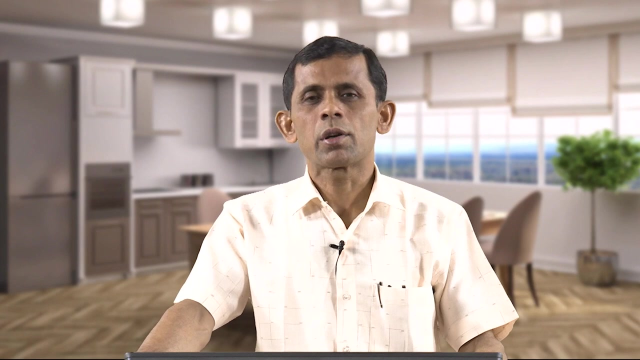 to reduce the environmental load. and that way the research is going on and technologies are being developed. So that is one, an introduction of treatment systems. So if it is there, that may have been some gases, say flue gas, desulphurization techniques. so for the separation of socks, 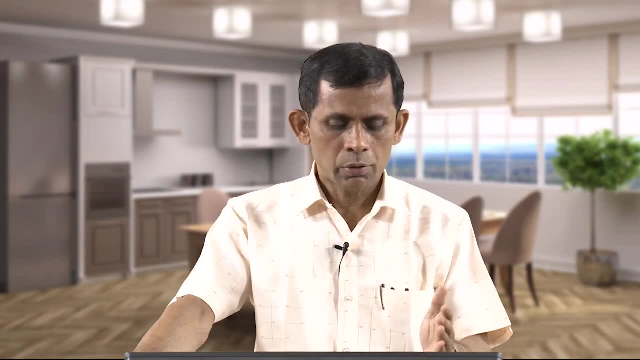 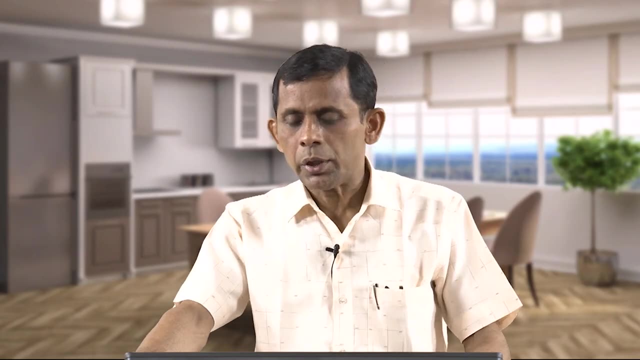 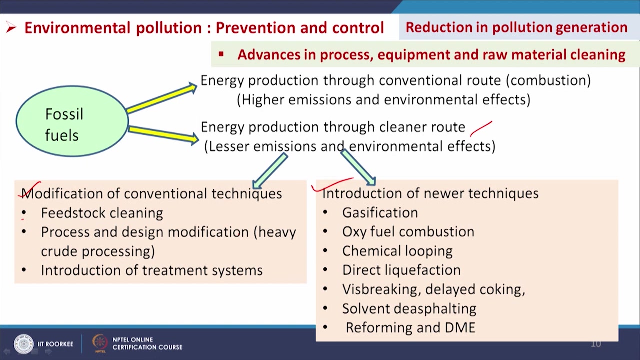 or separation of nox from the flue gas, So different. your introduction of treatment systems is possible to reduce the pollution. Another introduction of newer techniques like, say, gasification, oxy fuel combustion- I have given one example- and then chemical looping system, direct liquification of coal and 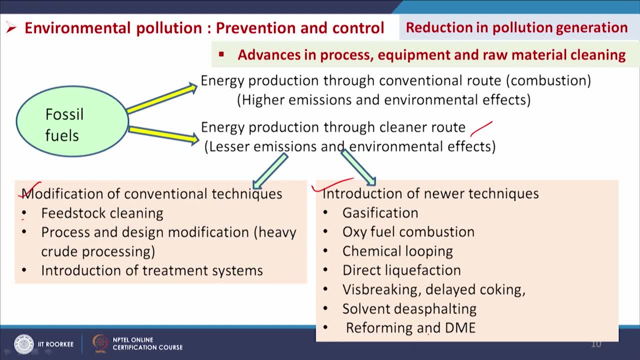 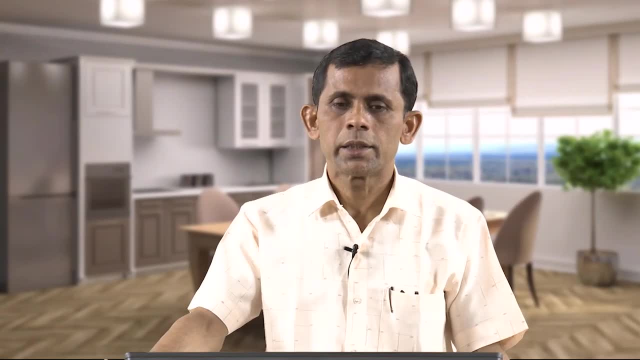 then vis breaking, solvent deasphalting. These three- beach breaking, delayed cooking and solvent deasphalting- are the residual upgradation of any petroleum refinery. And then we can go for reforming and DME synthesis, dimethyl ether synthesis, So natural gas can be reformed without going. 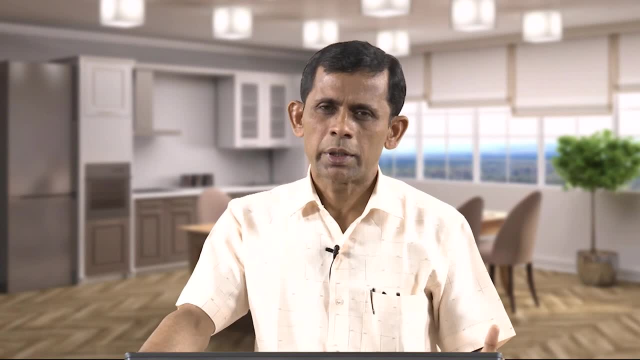 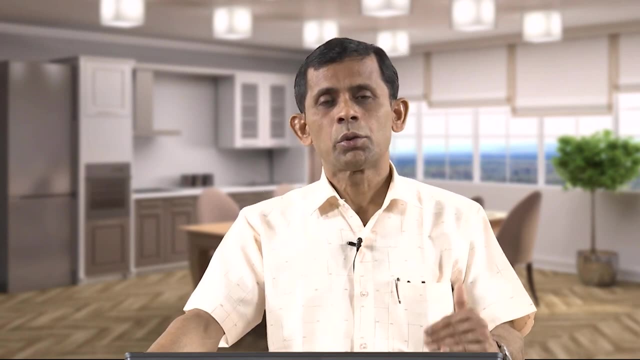 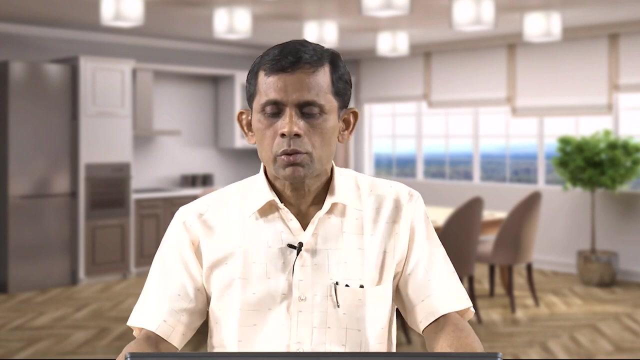 to your combustion route. We can. it can be reformed and then dimethyl ether can be produced. Once dimethyl ether can be produced, or hydrogen can be produced, so the carbon dioxide emission to the environment will be reduced, And this is another alternate sources of energy. 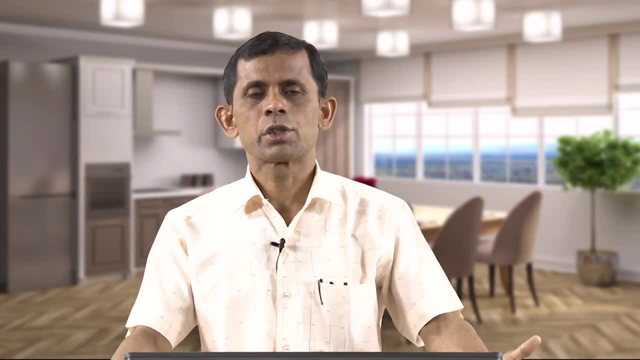 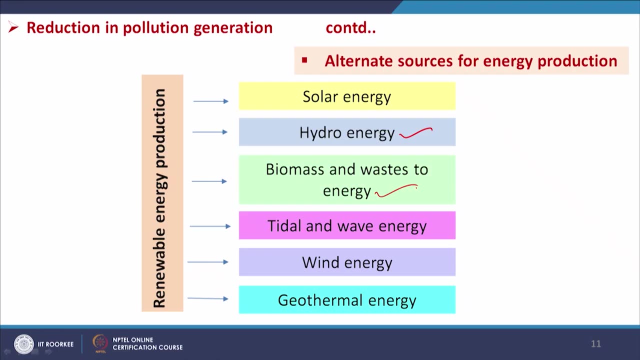 production. We can use other sources of energy productions in place of fossil fuel based energy, like, say, solar energy. we can use hydro energy. we can use biomass and waste to energy, and then tidal and wave energy and wind energy and geothermal energy. So these are the some. 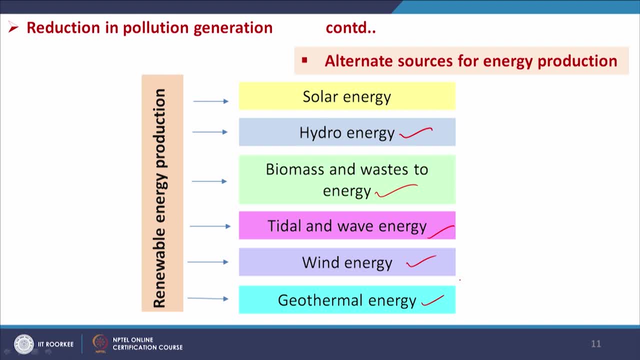 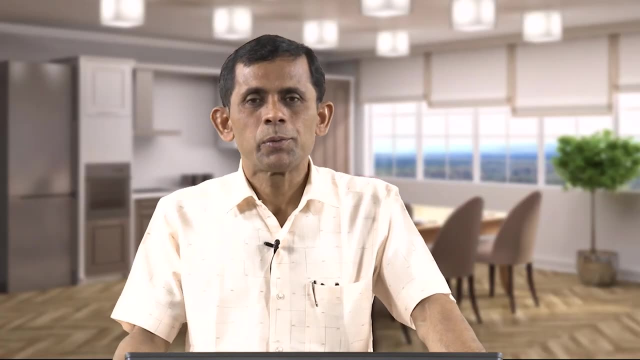 examples of renewable energy. So if we can produce energy through these routes and reduce the use of fossil fuels as a result, we will be able to save some environmental pollution. So pollution will be reduced. So that good practice. we have also talked about a good practice. One example here you 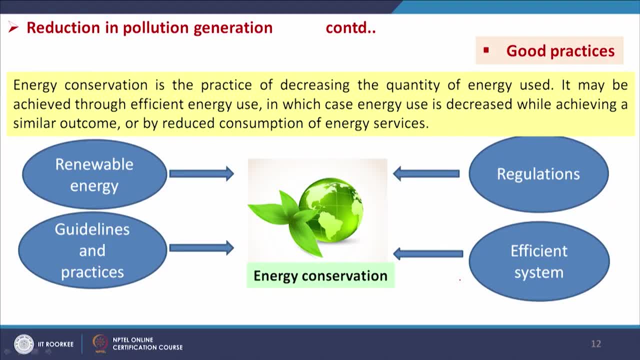 see that energy conservation. So what is this? Energy conservation is the practice of decreasing the quantity of energy used. It may be achieved through energy conservation. So what is this? Energy conservation is the practice of decreasing the quantity of energy used through efficient energy use, in which case energy use is decreased while achieving 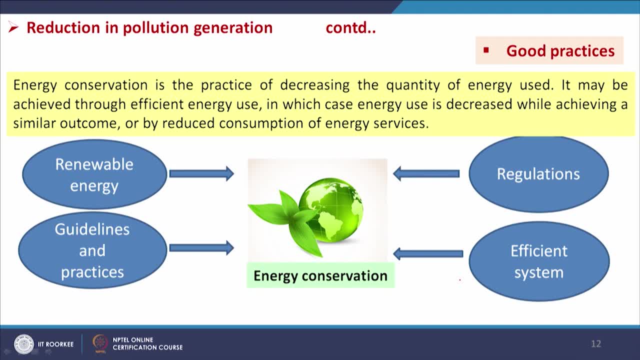 a similar outcome, or by reduced consumption of energy services. So this energy conservation is a technique or a practice. This can be achieved by different ways. One is efficient system. We can use efficient system so that the energy loss will be reduced. We can use 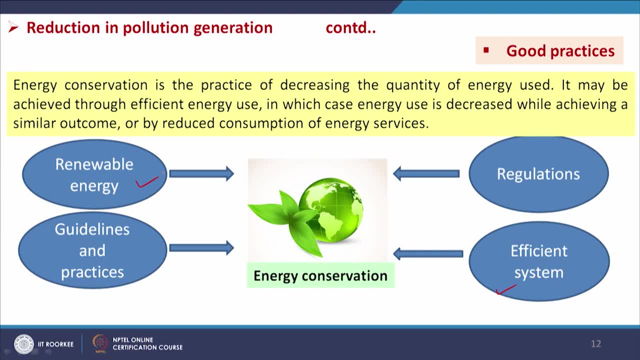 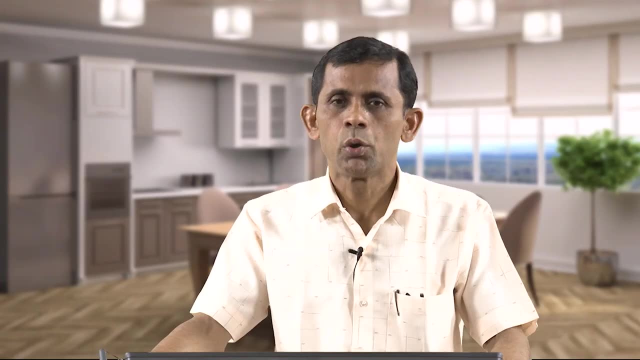 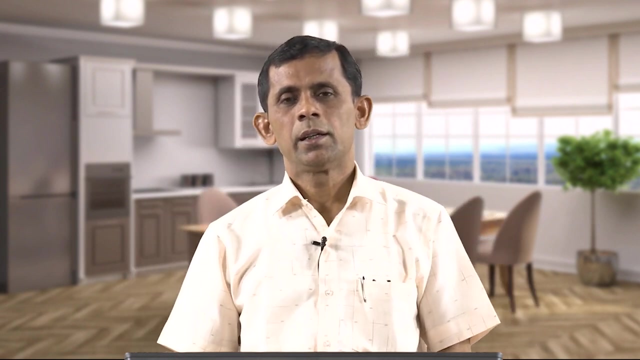 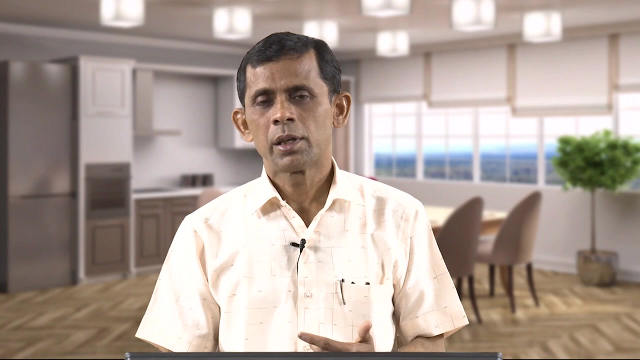 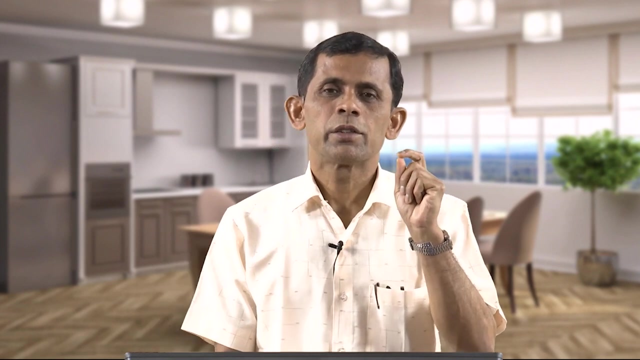 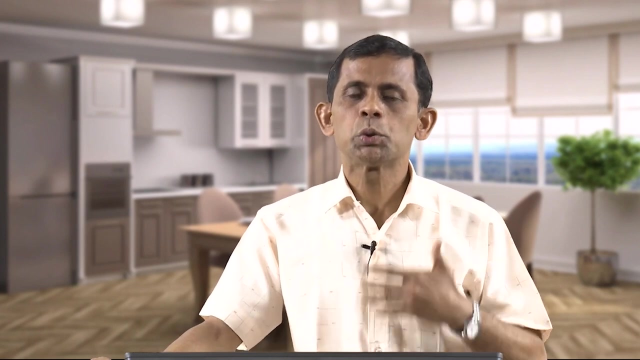 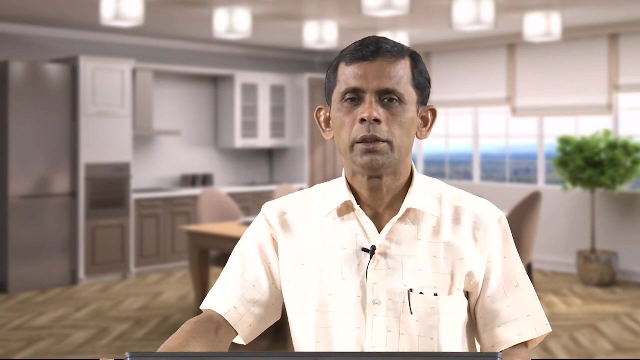 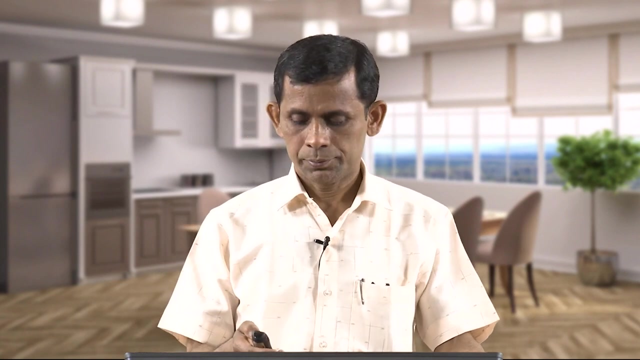 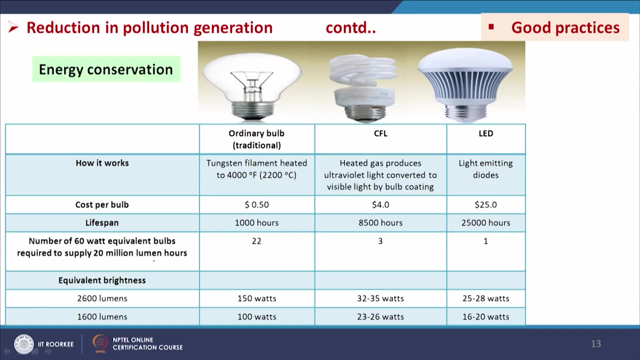 renewable energy, So energy conservation. here I am giving you some example. Say, we know that today we use the LED. prior to it, we used CFL. prior to it, we used ordinary bulb. So by the use of this technology and making it a practice, you see, initially we need to invest more. 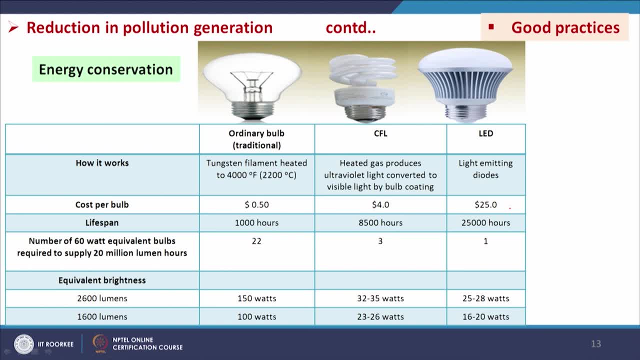 but ultimately we get the gain from all aspect, economically and environmentally. You see here what is the power requirement: 2600 lumens, same same energy consumption. So this is result: forrodinary bulb, and here we need to 32 to 35 watts, and for LED we need 25 to 28 or watts. 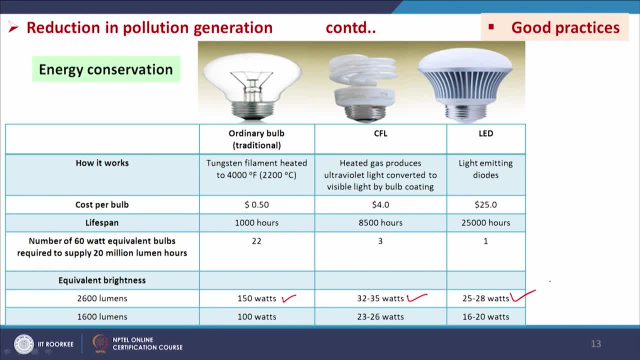 So, as result, we are using very less amount of energy to get the same impact. So initial investment is higher, but we are able to shave the environment by reducing environmental pollution and consuming lesser energy. So can you more or less, then, cafe truly contribute? 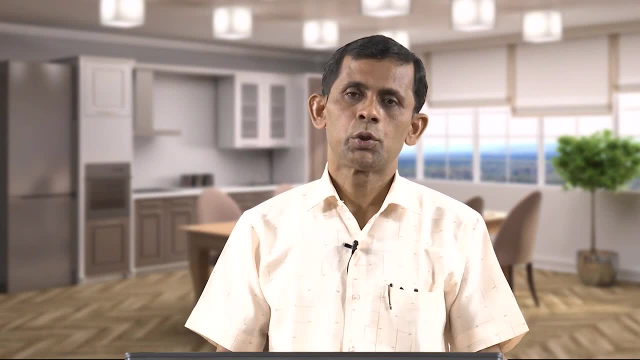 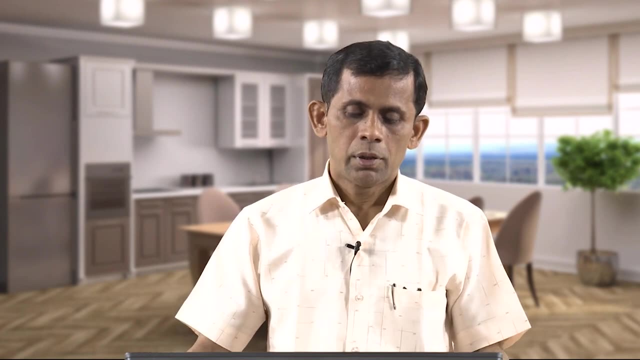 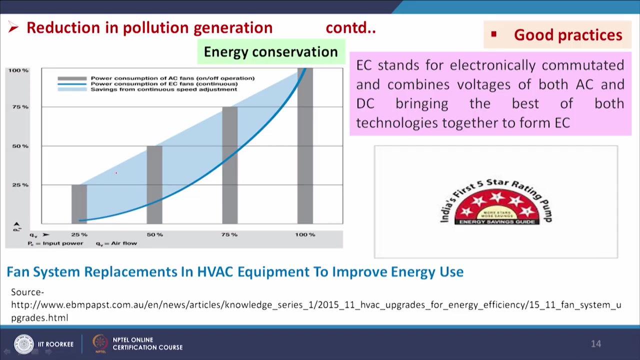 lesser energy, So that way this practice can help to improve the environmental quality. Similarly, the fans there may be on off operation or may be continuous operation. If we go for continuous operation, so then we will see that we can save this amount of energy. This. 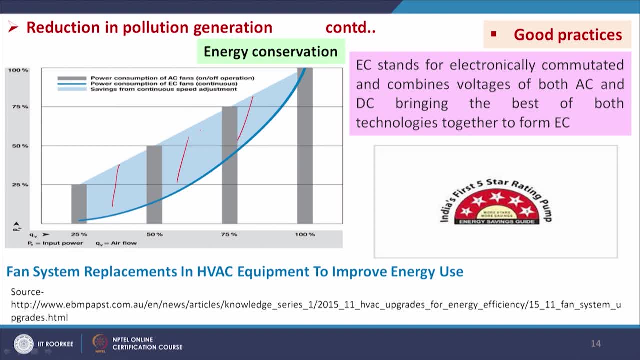 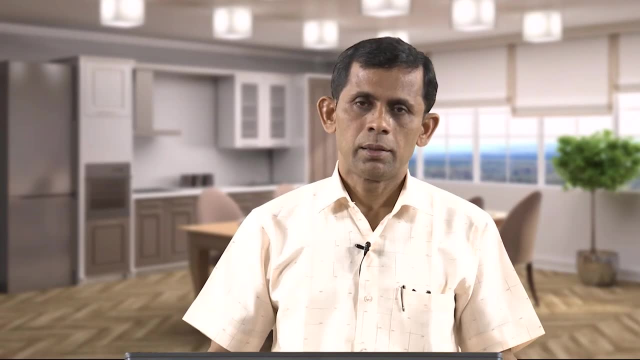 is for continuous operation, this is for on off operation, So that is also practice. We can purchase only 5 star rating electrical appliances, So the energy consumptions will be less than the other one. So these practices will help us to get the environmental quality. 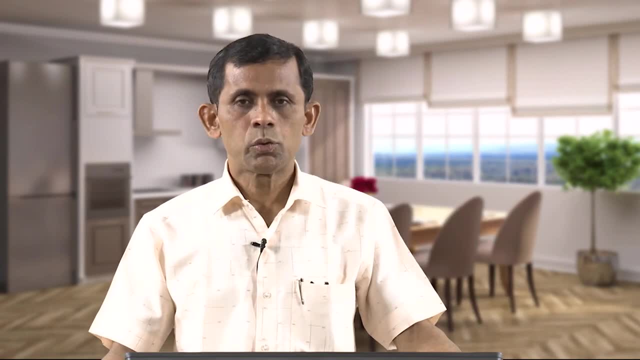 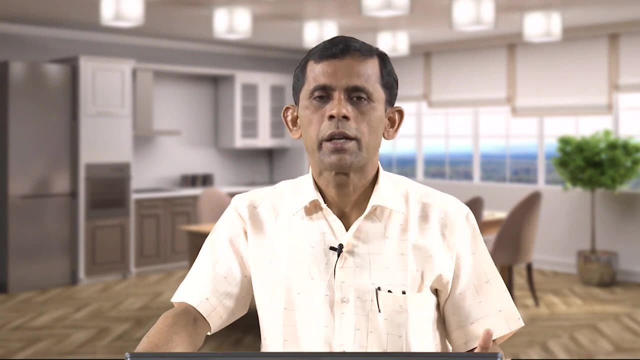 And then we are coming to the treatment. So waste water treatment: we can do the waste water treatment that there are primary, secondary, tertiary treatment methods are there and through which we can reduce different types of pollutants present in the waste water, As example, say, 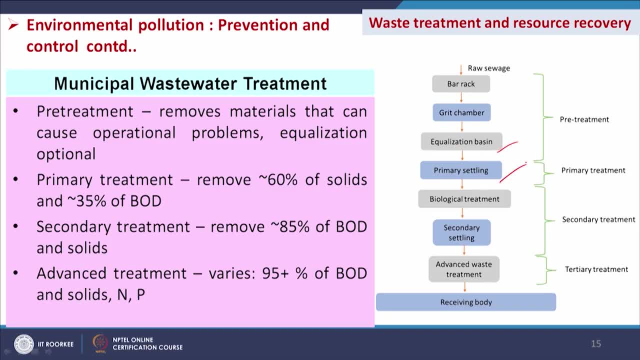 here barrack, Then grit chamber, equalization tank, primary settling, biological treatment, secondary settling, advanced treatment and ultimately receiving body water. the treated water we can use for other application And we see the primary treatment. it removes 60 percent. 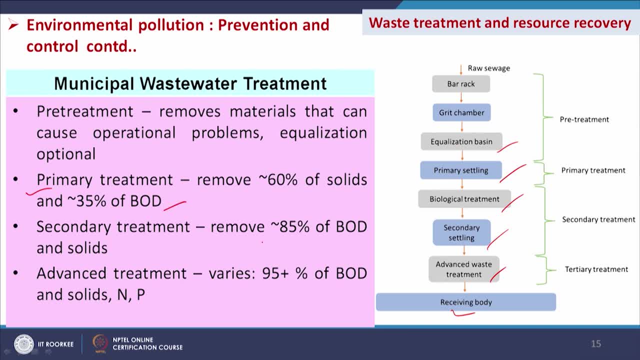 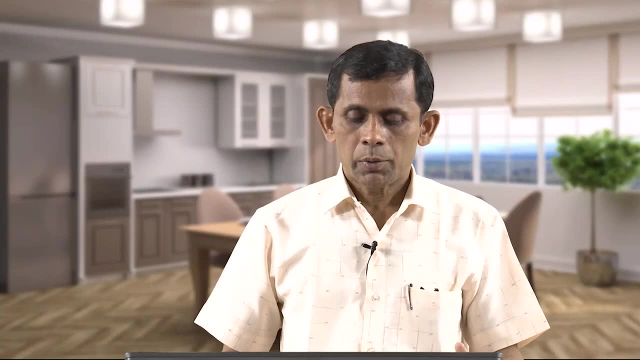 of solids and 35 percent of BOD, and secondary treatment remove 85 percent of BOD and solids, and advanced treatment varies 95 plus minus of BOD and solids. nitrogen, phosphorus, all those things are removed by this treatment methods So we can develop techniques for the municipal solid waste management that is, you know, segregated. 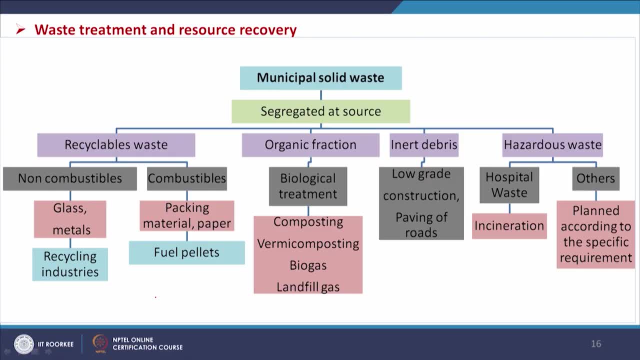 segregation of the waste at the source. that can be into segregated into different fractions. that is, recyclable waste may be organic, fractions may be inert debris, may be hazardous waste and all those fractions will be managed in a different way, like, say, non-combustibles. 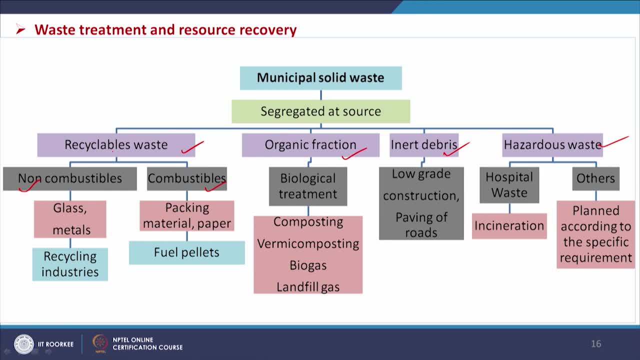 and combustibles out of the recyclable waste. If we have, then those will be managed in different way. For non-combustible waste we have non-combustible waste and non-combustible waste. non-combustibles glass metals like that- that will go through the recycling. 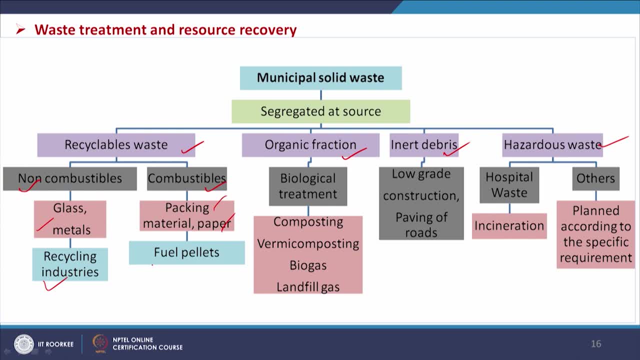 And this packaging materials, papers. this combustible materials can be converted into fuel pellets and it can be converted into energy and organic fractions. biological treatment: it can be processed through and composting, vermicomposting biogas landfills. these. 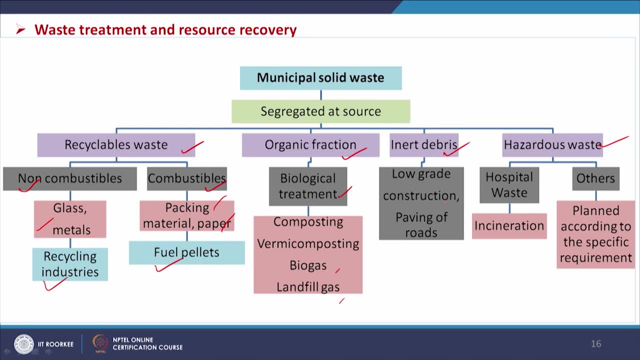 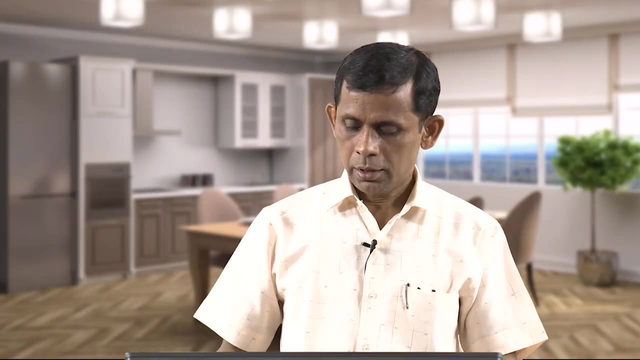 are some methods which can be used. Inert debris can be used for low grade constructions and paving of roads, and then hazardous waste, that is, hospital waste and others, may be processed in, as per the quality and the quantity of these wastes. So we will be discussing in detail about all those things and, as I told you, that waste. 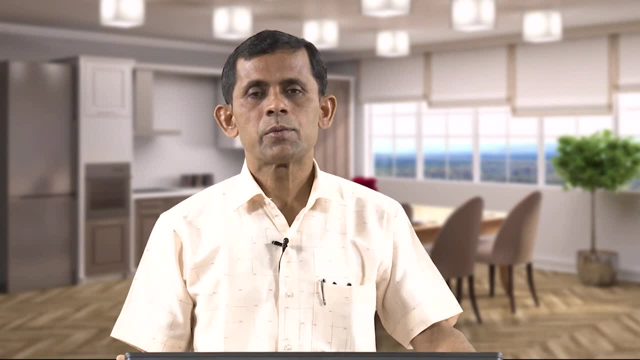 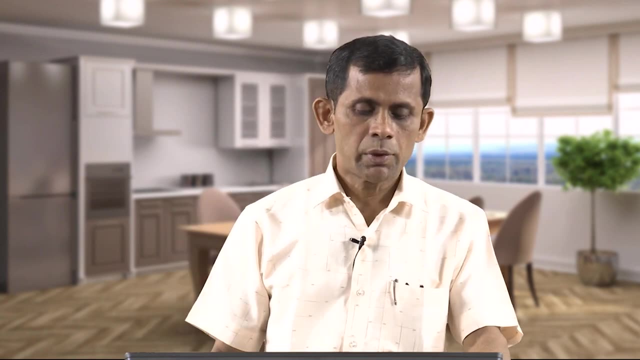 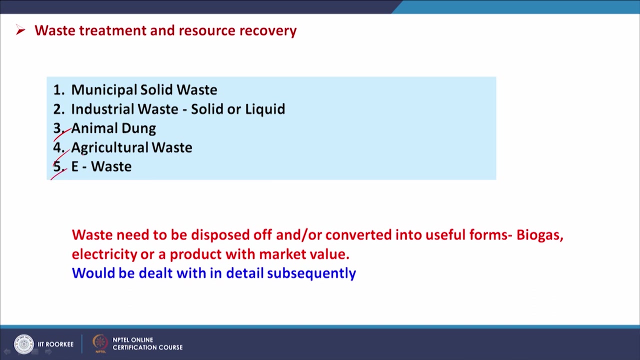 to wealth and waste treatment and wealth recovery is becoming a new concept and people are putting more effort to recover wealth from the wastes. So municipal solid waste, industrial solid waste, animal dung, agricultural waste, e-waste- all are being investigated to produce valuables. 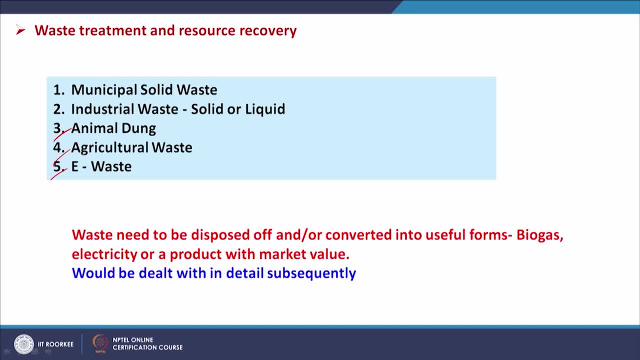 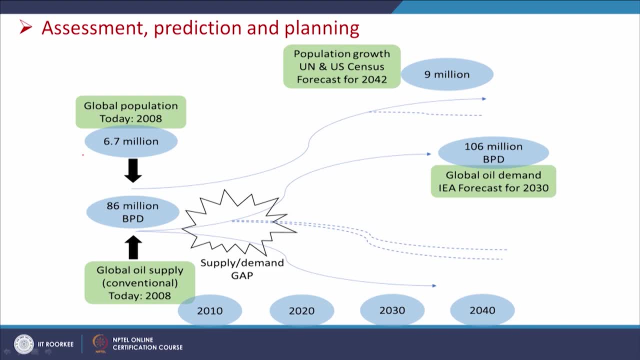 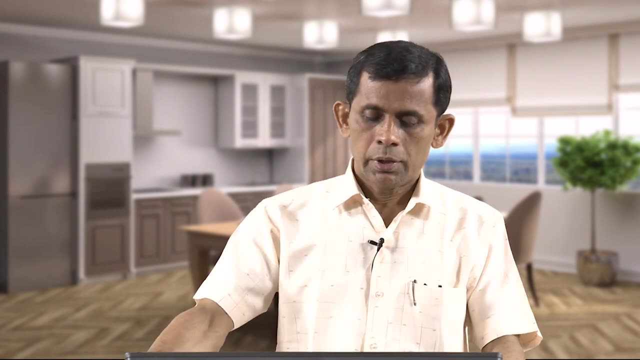 from it. So the state has to be responsible for this and the state has to be responsible for that, because we have to be responsible and the state has to be responsible for all the things which are planned, and that is why they have to be called the national climate education system. 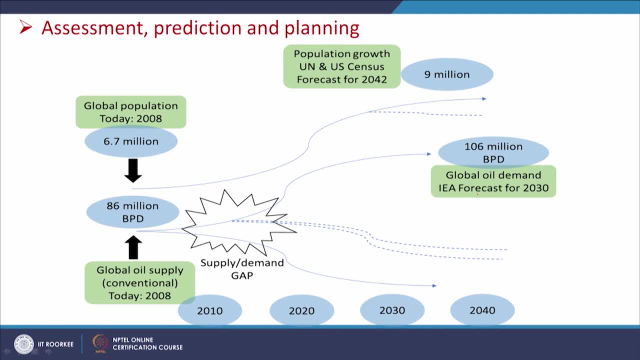 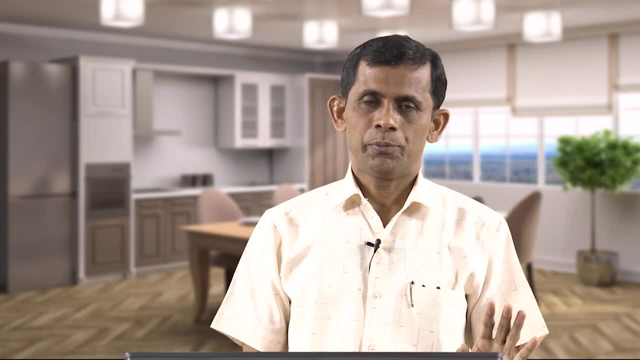 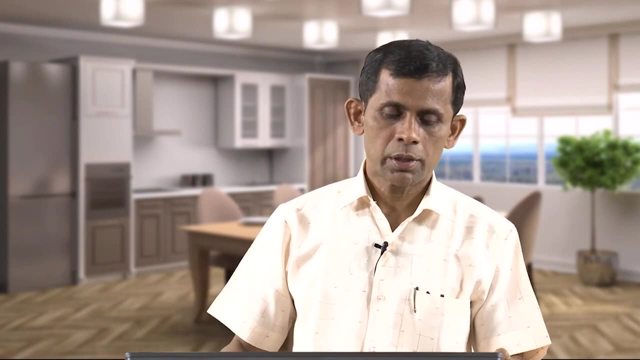 it is a national climate education system. So the state, So that is all Okay. So we also need to take decision and planning for our future environment, clean environment, For example. you see national solar mission, national mission on enhanced energy efficiency. 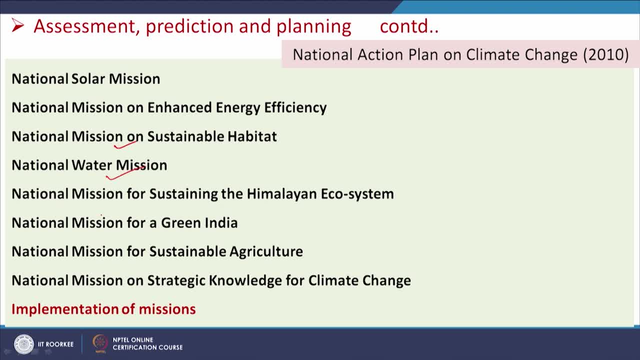 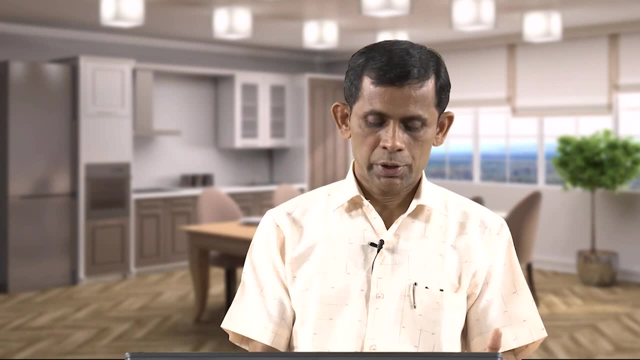 national mission on sustainable habitat, national water mission, national mission for sustaining the Himalayan ecosystem, national mission for a green India, national mission for sustainable agriculture, national mission on strategic knowledge for climate change, and another is implementation of these missions. Missions: we can mix, we can develop some missions, but the implementation is most important. 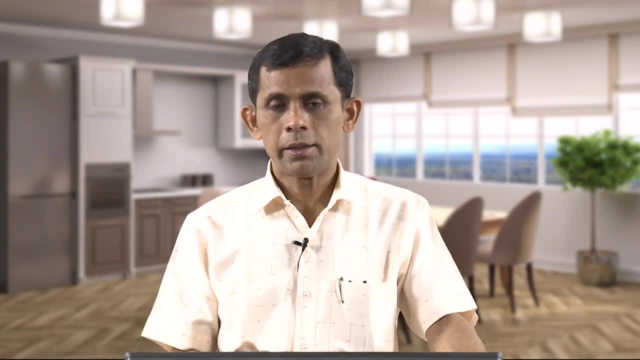 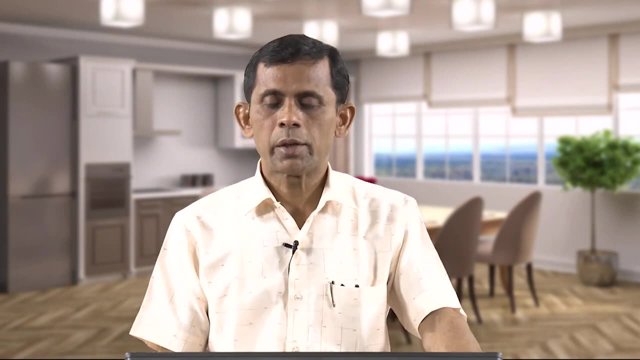 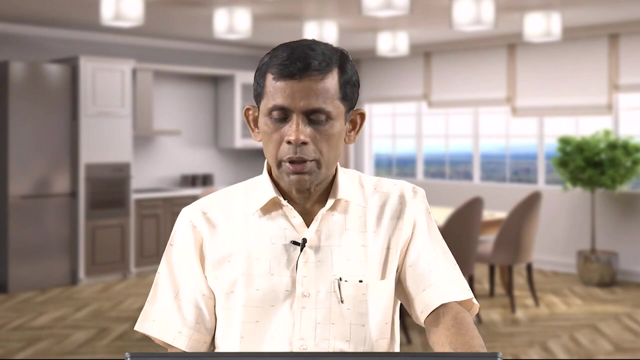 So that is also we have to do to ensure the clean environment. Now, just I will give you some glimpse of the Joharlal Nehru national solar mission in 2010.. It was established And then the target was To make 20,000 megawatt of solar power by 2020, and there are some interim assessment. 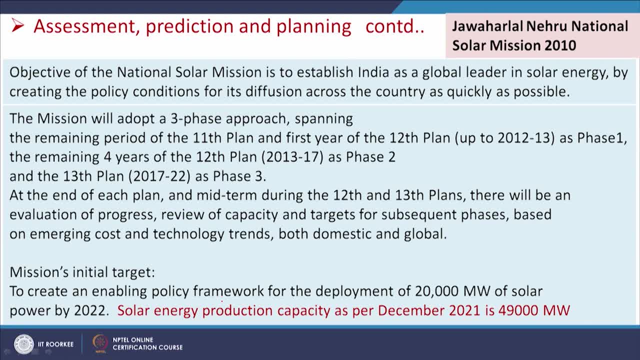 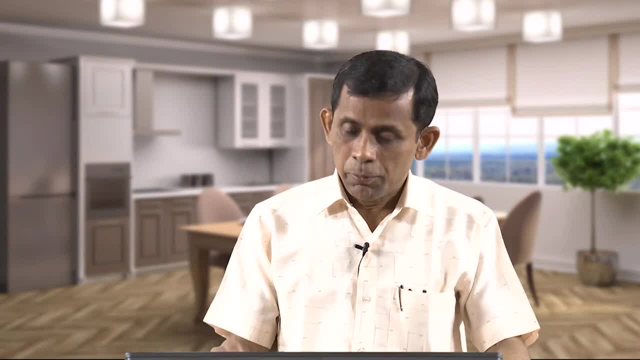 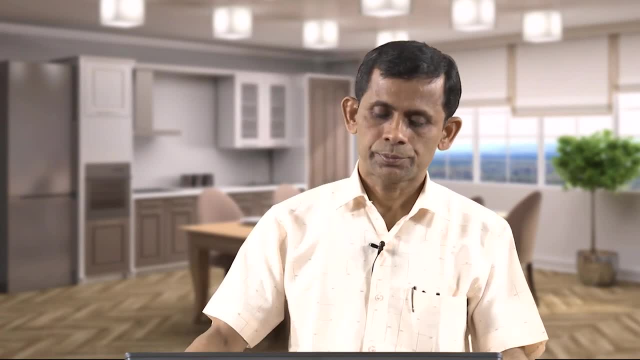 options were also there. but you know, we are very happy to know that this mission got success and before 22, in December 2021, 49,000 megawatt solar energy is produced in the country. So this is installed capacity and December 2021. 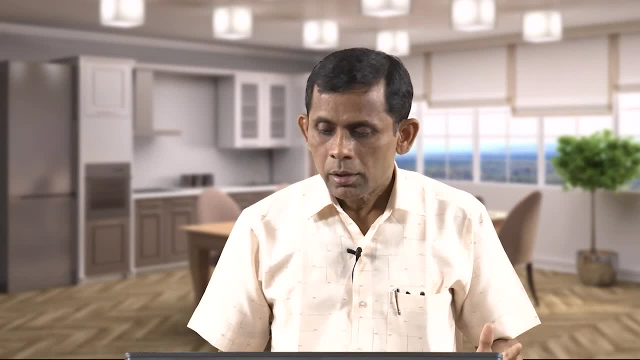 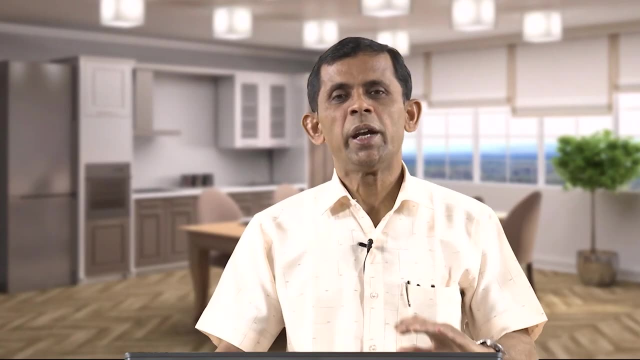 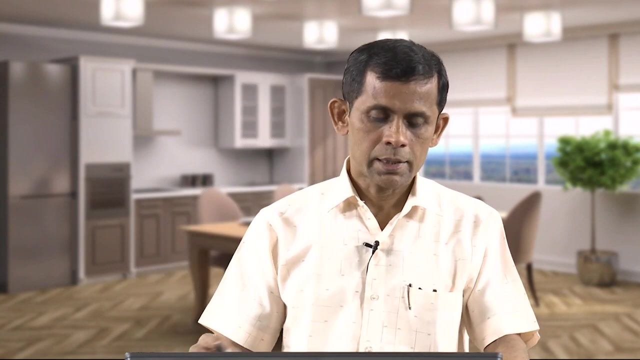 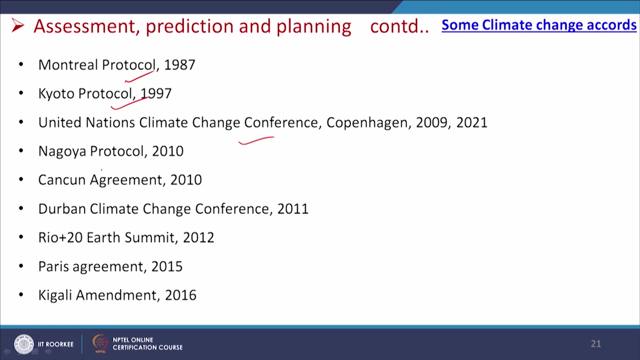 So, similarly, You know, many international accords or treaties are also done to maintain the climate change, to protect the climate change across the globe, Like, say, some examples are Montreal Protocol, Kyoto Protocol, United Nations Climate Change Conference, and then Nagoya Protocol, Can-Can Agreement, Durban Climate Change Conference. 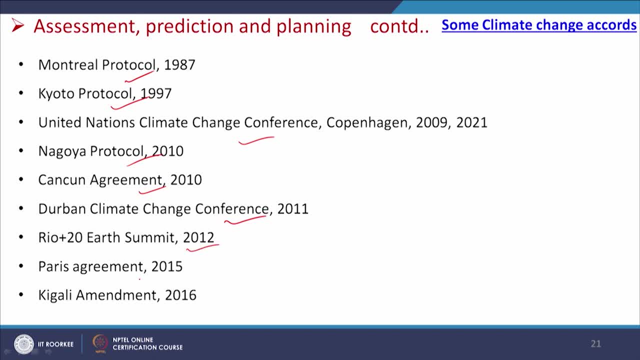 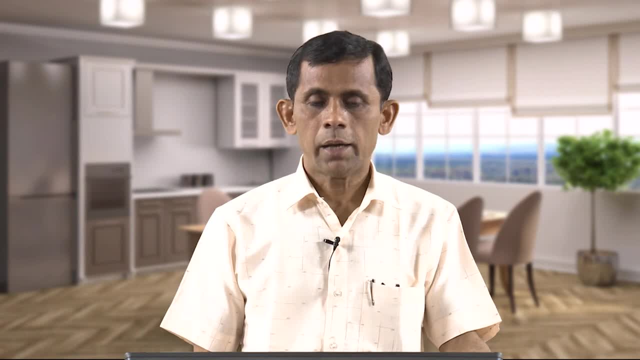 Rio 20 Earth Summit and the World Climate Change Conference. So these are some examples. So these are some examples. So these are some examples: Paris Agreement, Kigali Amendment. So these are some accords which are related to the climate change, and then we need one. 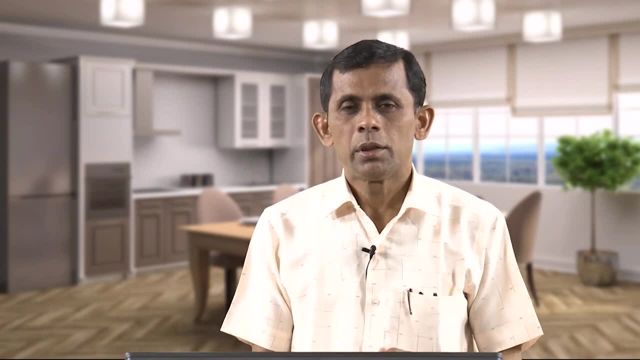 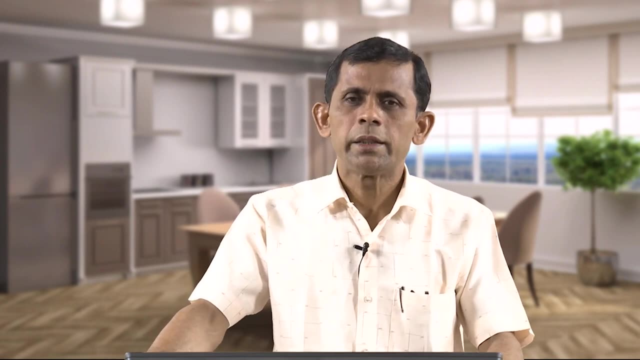 framework and we should have good ethics on the environment. Each individual should be responsible to maintain the environmental quality through their different activities. That is very essential. We have to make the people aware about it And each organization should take responsibility to maintain the environmental quality through. 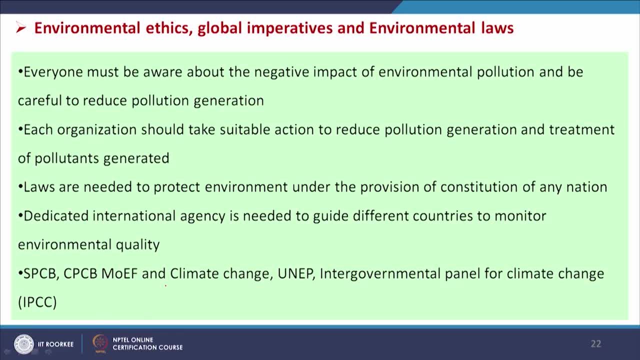 their different activities. That is very essential- take suitable action to reduce pollution generations and treatment of pollutants generated, and laws are needed to protect environment under the provision of constitution of any nation, and dedicated international agency is needed to guide different countries to monitor environmental quality. and all these are in existence. 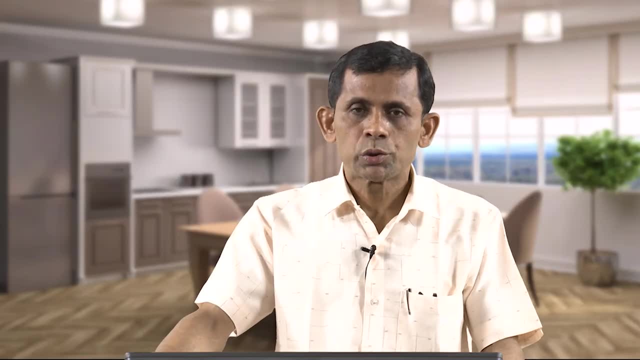 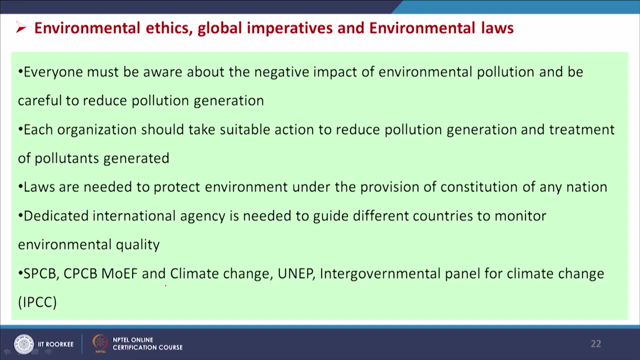 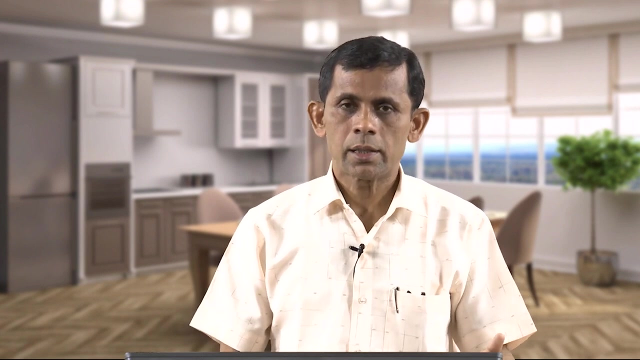 Like, say example, in our country we have state pollution control board. central pollution control board, CPCB or central pollution control board is working under the ministry of environment and forest and climate change, UNEP, United Nations environmental program and intergovernmental panel for climate change, IPCC. these are also organizations which are working international. 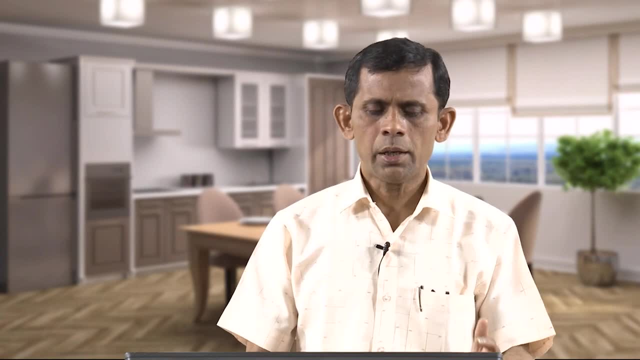 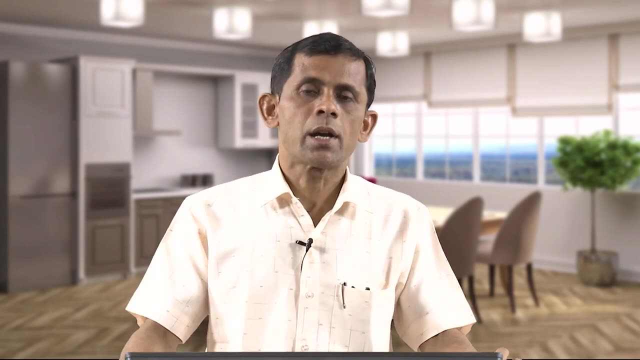 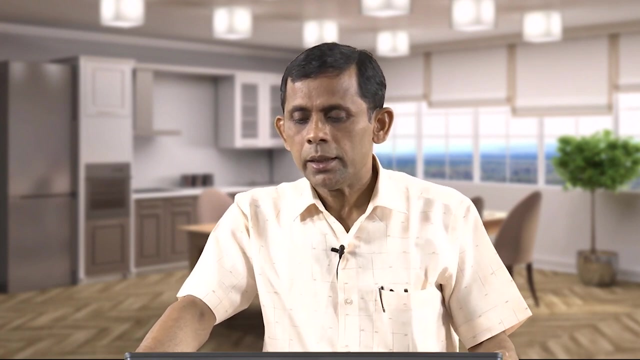 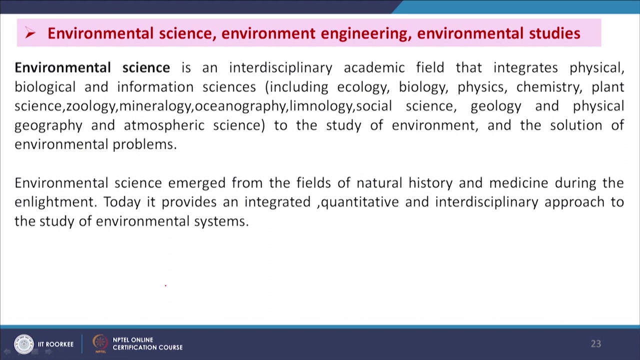 level to maintain the environmental quality. Now, at the last, we will see the what the environmental science, environmental engineering and environmental studies are. So environmental science is an interdisciplinary academic field that integrates physical, biological and information sciences to the study of environment and the solution of environmental problems. 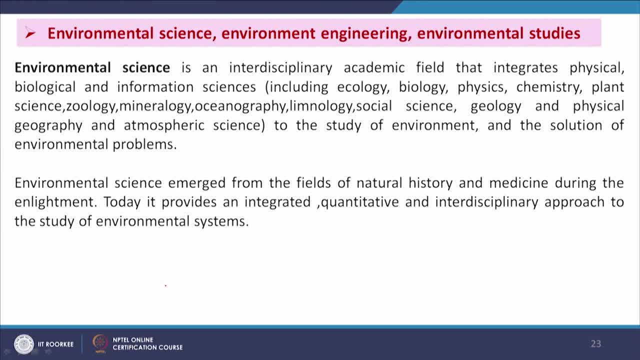 So it includes ecology, biology, physics, chemistry, plant science, zoology, mineralogy, oceanography, limnology, social science, geology and physical, geography and atmospheric science. So environmental science emerged from the fields of natural history and medicine during. 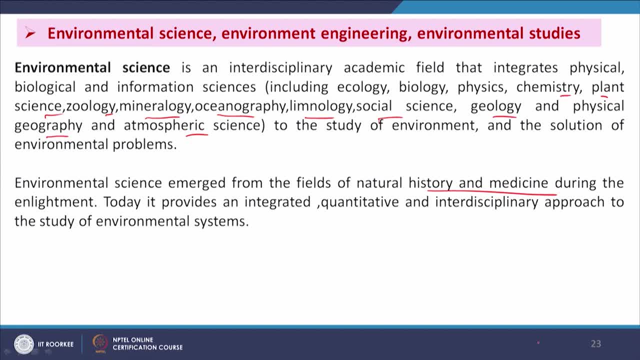 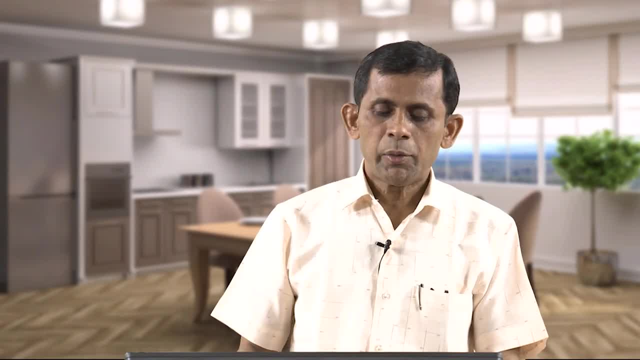 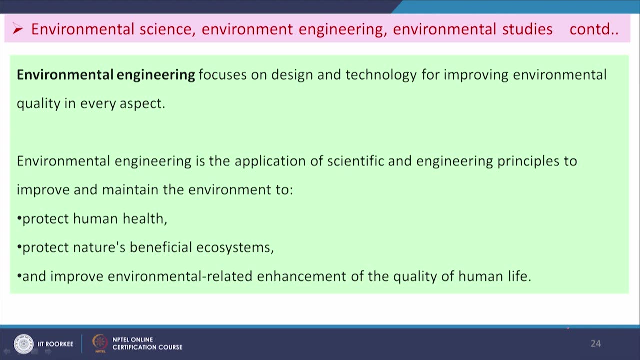 the enlightenment. today, it provides an integrated, quantitative and interdisciplinary approach to the study of environmental system, and environmental engineering focuses on design and technology for improving environmental quality in every aspect. Environmental engineering is the application of scientific and engineering principles to improve and maintain the environment, to protect human health, protect natures, beneficial ecosystem. 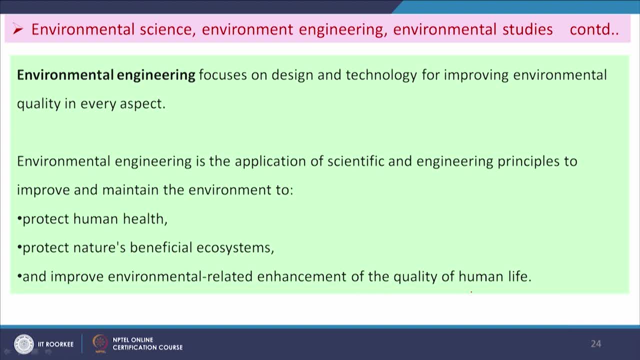 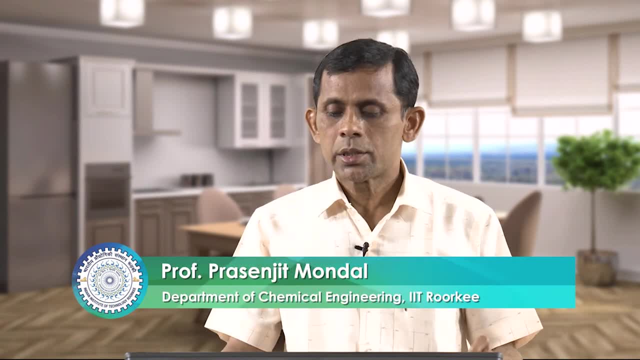 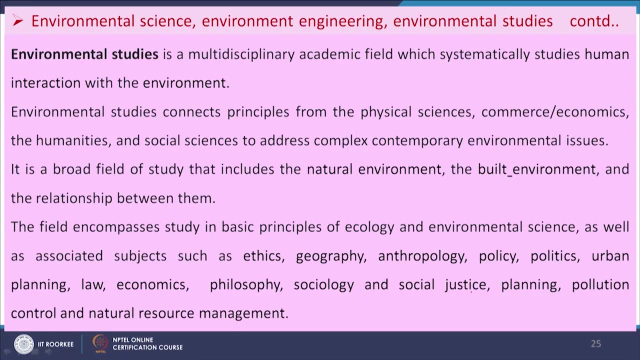 and improve environmental related enhancement of the quality of human life. and environmental studies is a multidisciplinary academic field which systematically studies human interactions with the environment. environmental studies connects principles from the physical sciences, commerce, The social sciences to address complex contemporary environmental issues. 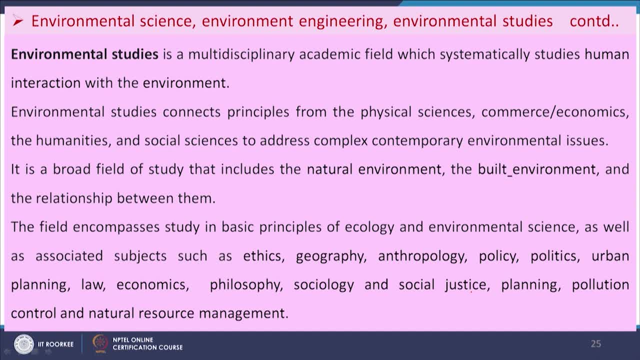 It is a broad field of study that includes the natural environment, the built environment and the relationship between them. The field encompasses study in basic principles of ecology and environmental sciences, as well as associated subjects such as ethics, geography, anthropology, policy, politics, urban development. 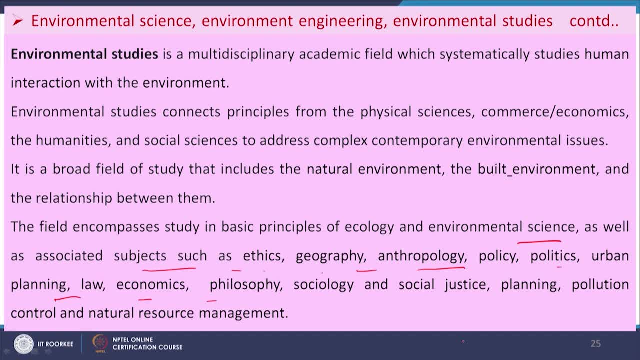 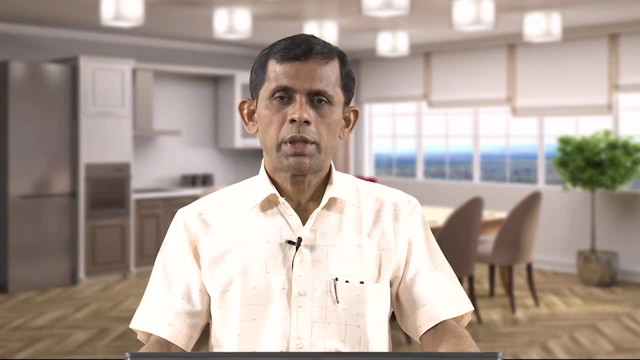 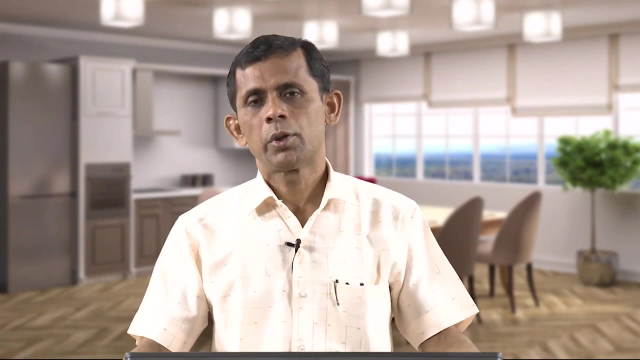 urban planning, law, economics, philosophy, sociology and social justice, planning and pollution control and the natural resource management. So these are the different subjects which we should know so that we can take proper action to prevent and control the pollution. Thank you very much for your patience. Thank you very much.